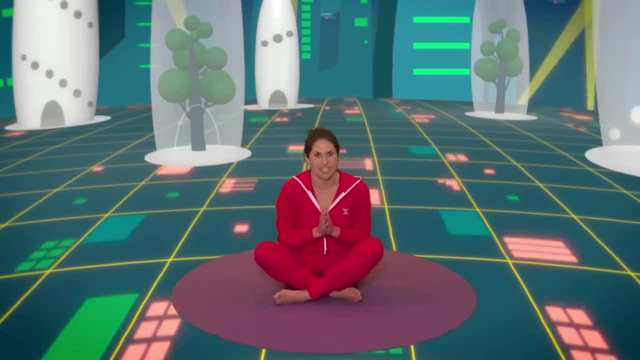 at our hearts and saying our secret yoga codeword, which is: Namaste Ready After three, One, two, three, Namaste. There, Now we're ready to begin, And today we're going off 100 years into the future to meet a very special dog called Sparks 24.. He's a robo dog, A dog. 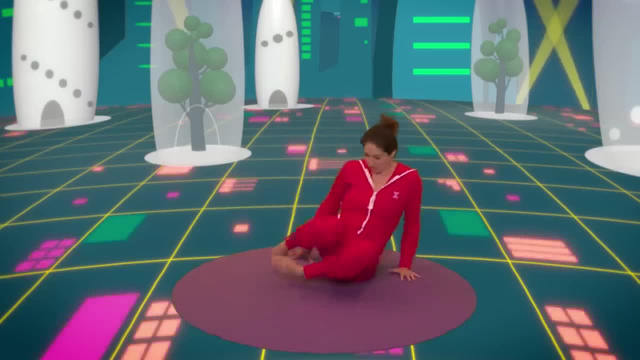 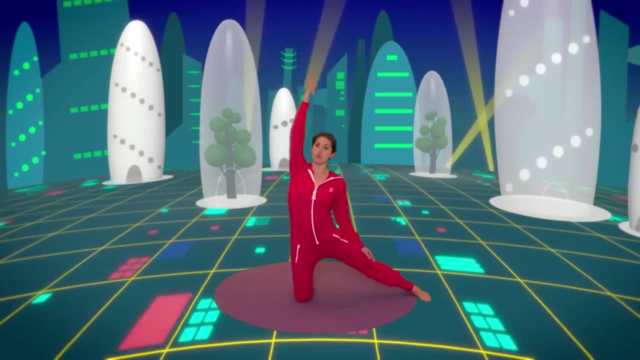 That's a robot, So we're going in a time machine. Coming up onto your knees And stick your leg out to the side. Lift your arm up to the air and let's open up the back door. Bring your knees back together again. Stick your leg out to the other side Now. 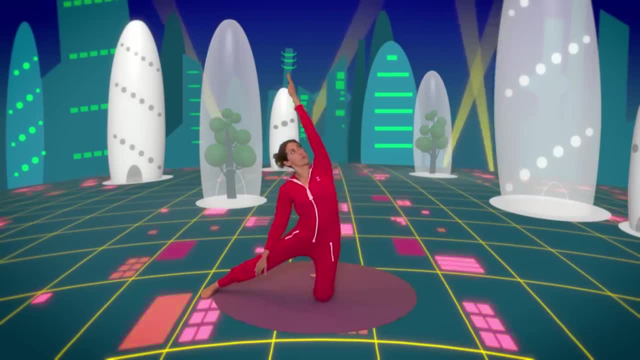 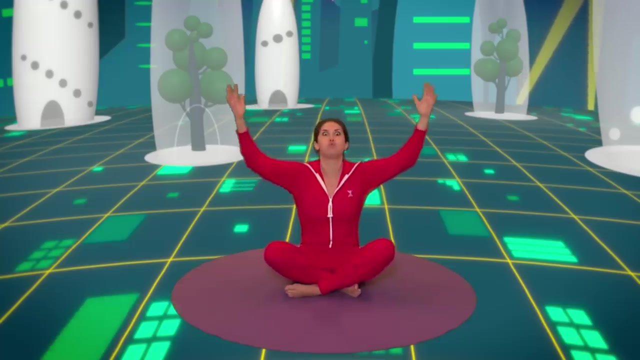 lift your other arm up and close the door behind you. Wow, Our time machine is a big round bubble. Cross your legs and blow your bubble up. I think that'll be big enough. Let's crawl inside, We come onto all fours and we reach. 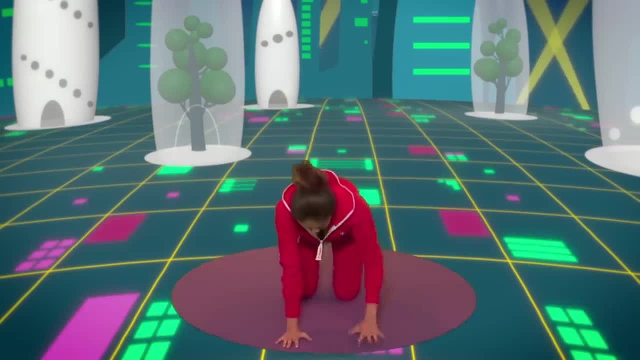 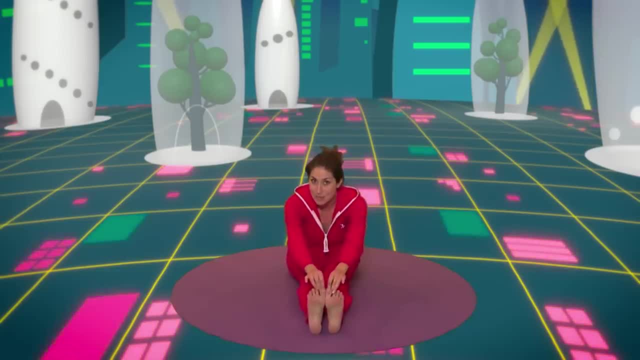 boop, boop, boop, boop, Setting the time for a hundred years in the future. We're ready for takeoff. Bend your knees, hands behind your bottom and let's lift our hips as we count down from five: Ready Five, four, three, two, one. Blast off Up, we go everyone. 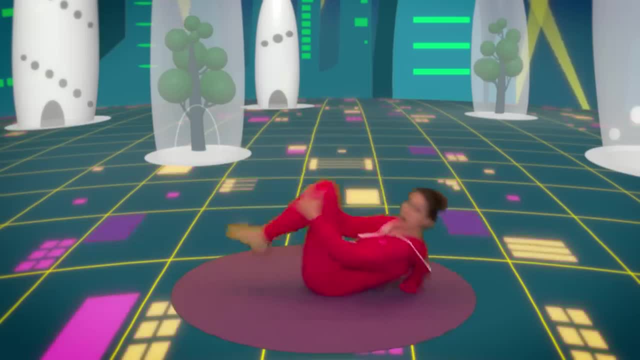 Legs up in the air. We're rocking, We're rolling, We're rocking And we're rolling. And then we go, very still, And we go from the side to the front, Ready To the other side, As we zoom through time forwards by one hundred years, we're coming. 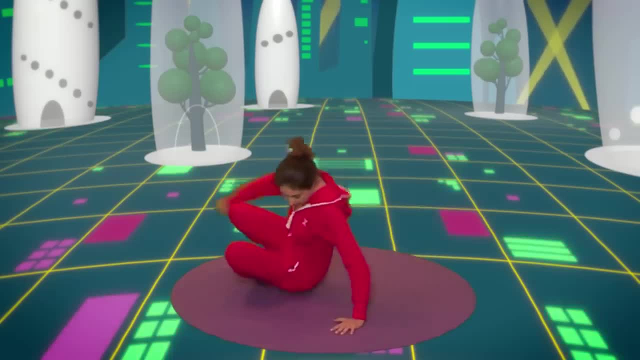 in to land, Coming onto your knees everyone and tucking up into a tiny little ball. We sit up and stretch. Wow, it's bright out here. We need to put on our eye protectors. Bringing your thumbs and fingers together, Pop the motion. 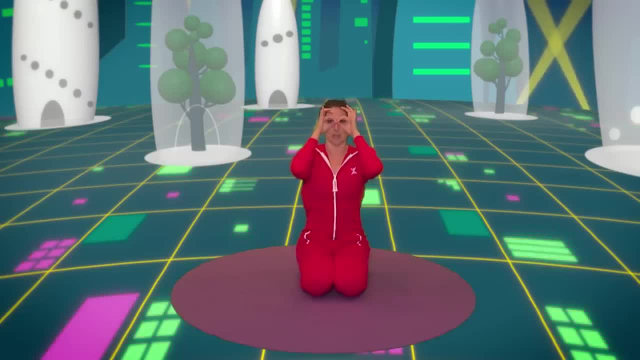 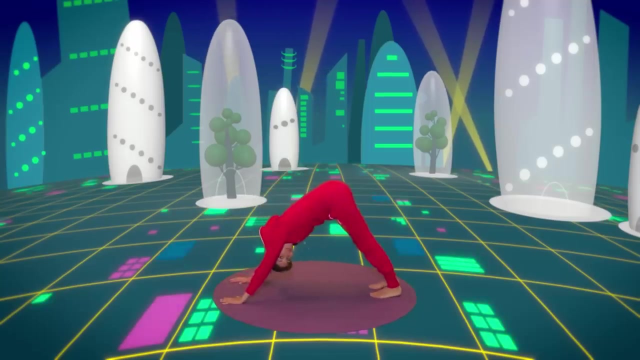 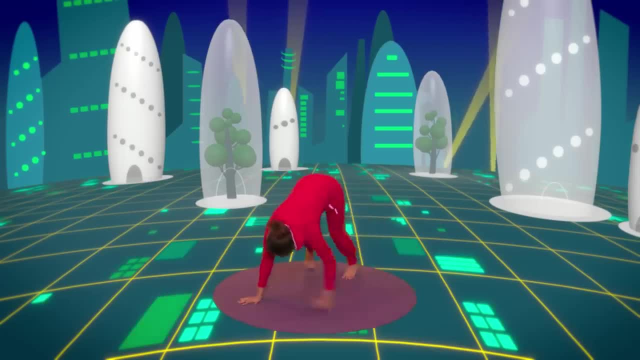 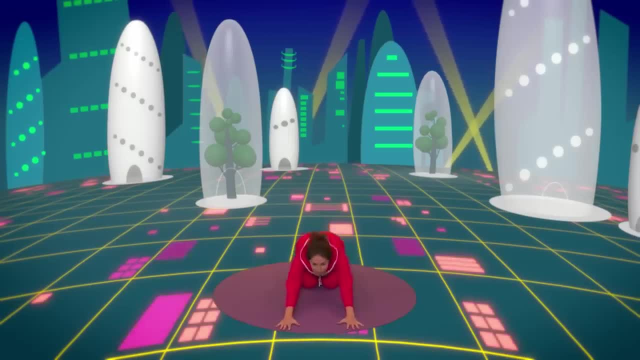 pant Woof, woof, woof, woof, woof, woof, woof. He's got two tails Coming up onto all fours. he lifts up one tail and gives it a wag with a little pant. Woof, woof, woof, woof, woof, woof, woof. 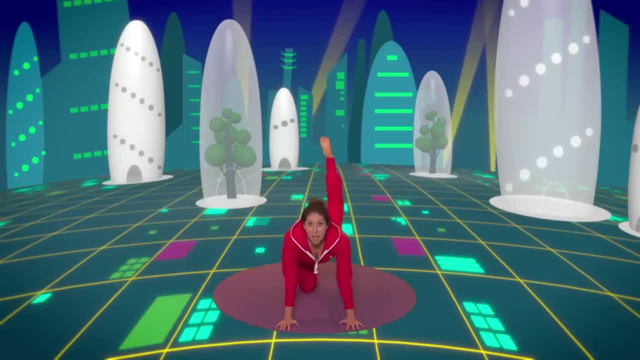 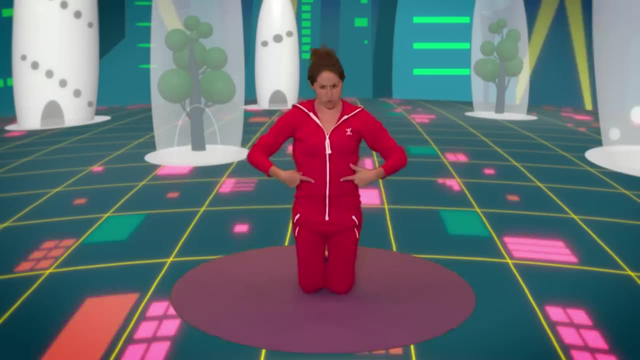 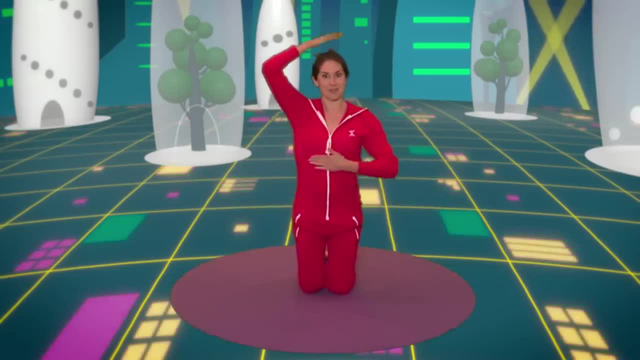 Now rubbing a hand around on your tummy. can you pat your head at the same time? Yes, you can, Sparx 24 says. When my tummy turns from green to red, it means that some part of my body has switched. 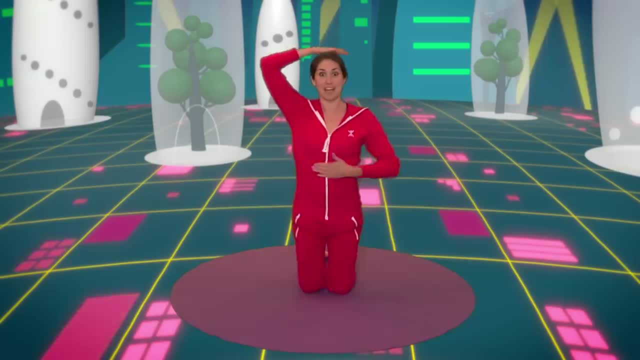 off. I need your help to help me switch myself back on again. You will hear a funny noise. Well great, Now we know that we can get on and explore the future. We get into a flyer. We get into a flying car. 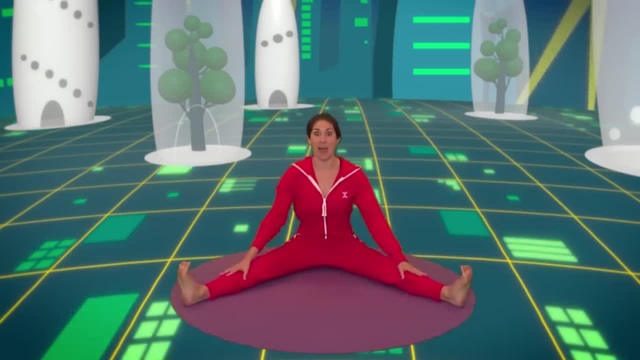 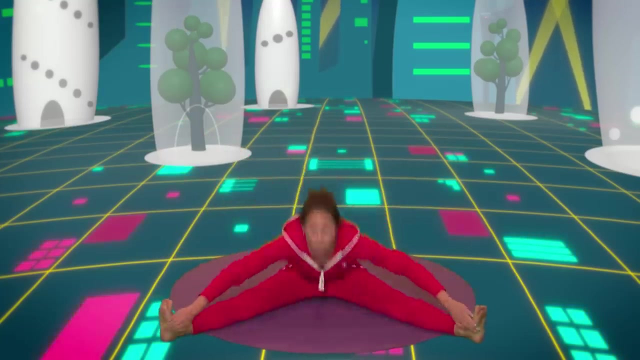 Put your legs out nice and wide. Wow, it's so cool As we flip over one side And then we flip over the other side, We go all the way back. up a hill, Wee, And down a hill, Wow. 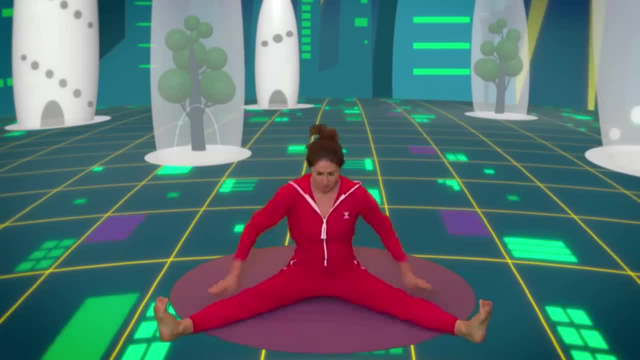 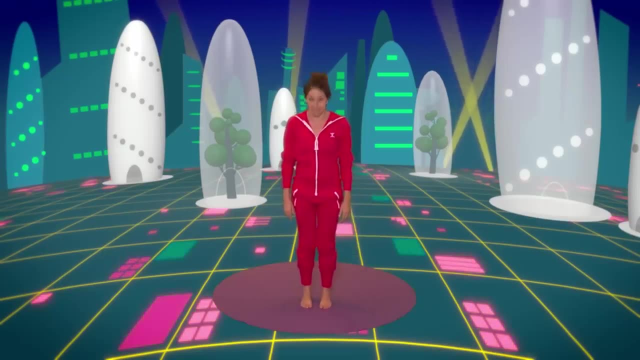 What a fun flying car, But we haven't seen much of the city. We get out and we look around. Wow, There are so many tall buildings. Jump your feet wide, Bring your hands up above your head. They've got very pointy glass roofs- Wow. 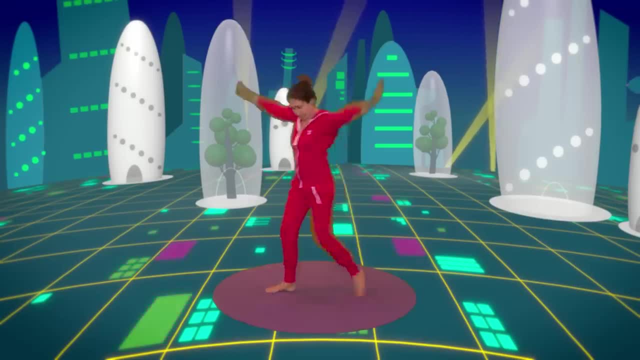 There are also lots of rivers in this city, with lovely little bridges sitting on your bottom, Put your hands behind your bottom and lift yourself up. We look in the water and we see there are lots of fish and they all have lights on their heads. 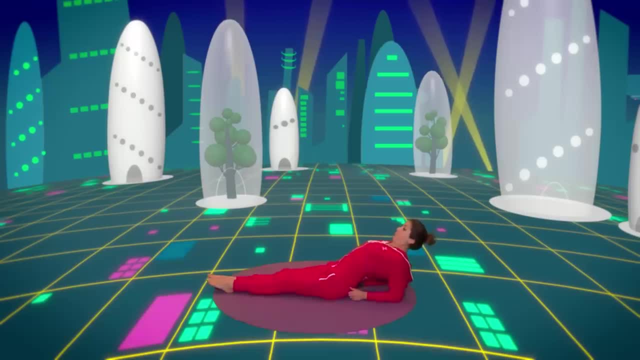 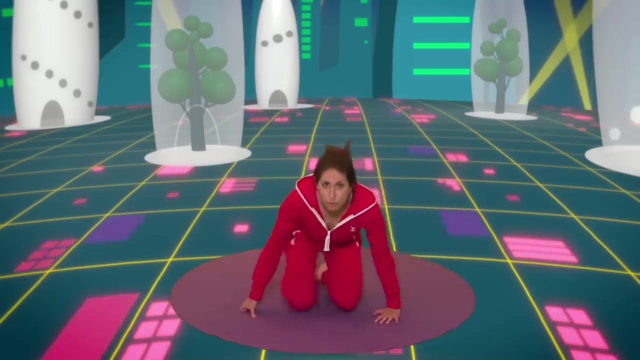 Point your toes down, Come down onto your elbows and pop, pop, pop your chest up and look all the way up And behind you. Wow, What amazing fish. All of a sudden, though, we hear a funny noise. Oh no, Sparx24's tummy has turned from green to red. Some part of him has switched off. 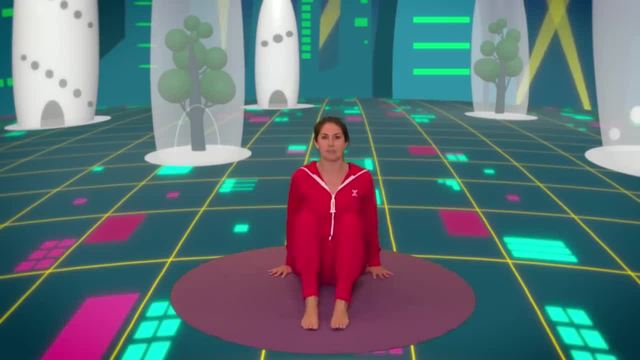 Let's do the check Sitting on our bottoms. we check his back paws. Lift them up. Yes, they still go side to side. What about his front paws? Yes, they still go side to side. What about his front paws? 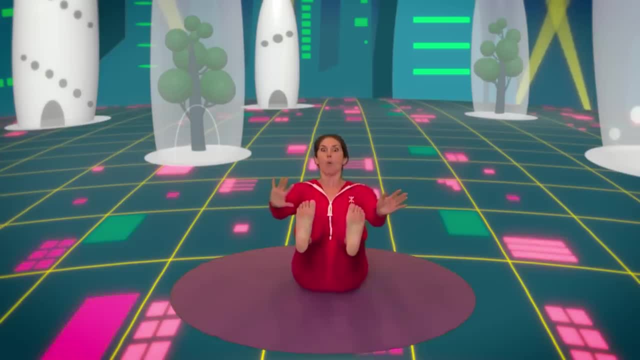 Yes, they still go side to side. What about his front paws? Yes, they still go side to side. What about his back paws? Yes, they still go side to side. What about his eyes? Yes, they still go side to side. What about his eyes? 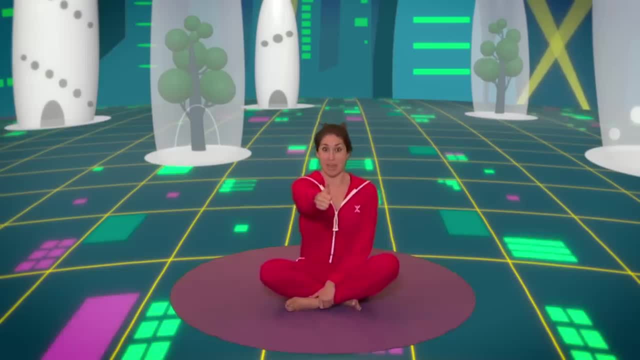 Yes, they still go side to side. What about his eyes? Cross your legs. Stick your thumb out Now without moving your head. see if you can follow your thumb with your eyes Up Down Side Side. Yes, 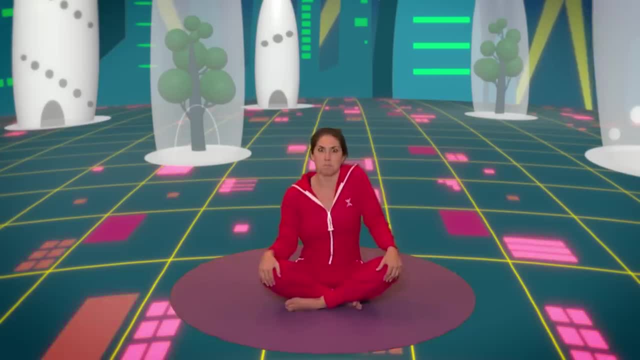 They still work. Maybe it's his shoulders. Can we lift up one shoulder, Two shoulders? Drop the first shoulder And the second shoulder Going up, Up, Down, Down, Up, Up, Down, down, up, up, down, down, up up. Yes, you can, Wonderful. 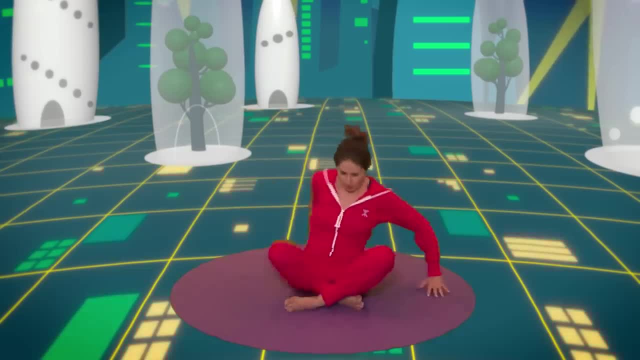 His shoulders are fine. Maybe it's his ears Coming on. to all fours We say Hello Sparks 24.. Oh, we don't hear anything. So it's his ears Sitting back. give your ears a rub right from the bottom. 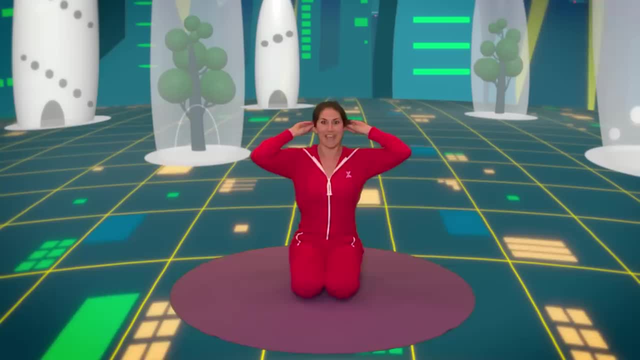 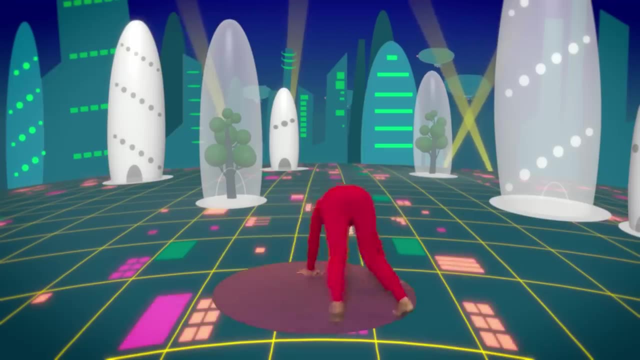 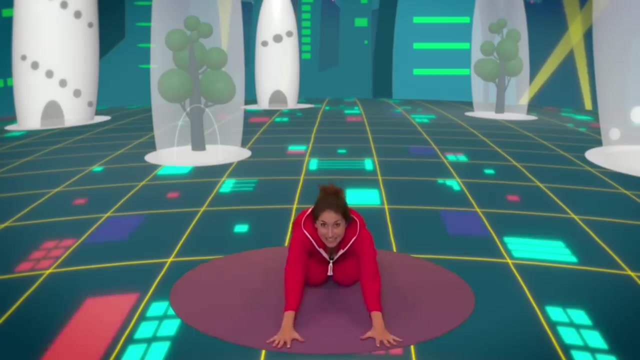 right the way around to the top to switch them back on again. Sparks 24 can hear again. He does a little spin, Comes down onto his little legs and stretches out his front paws to say Thank you. We're feeling quite peckish now. 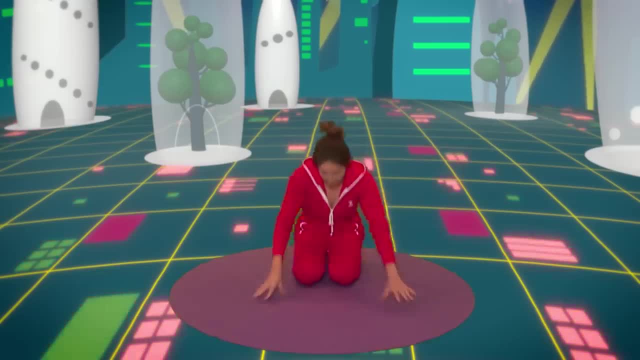 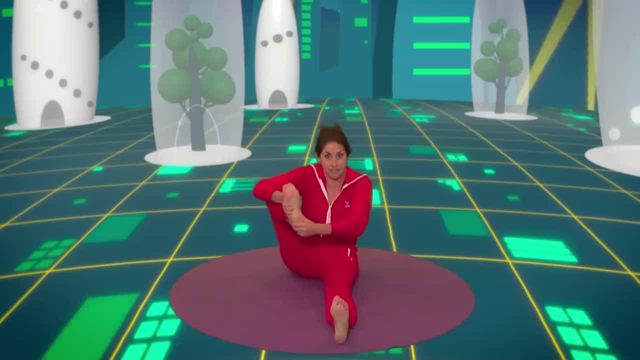 Sparks 24 says that we have to ask for what we want and we must say: please, Right, Oh, hello, Can I have a strawberry yoghurt please? Oh, coming right up, Thanks, OK, bye. Great, That's exciting. 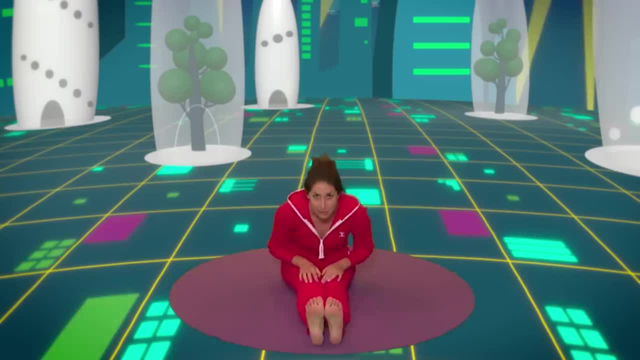 Now, apparently, when the other one rings, we have to say thank you, And that means we get our food in our mouths immediately. Ring, ring, Ring, ring, Ready, Hello, Oh, thank you, Oh, Mmm. 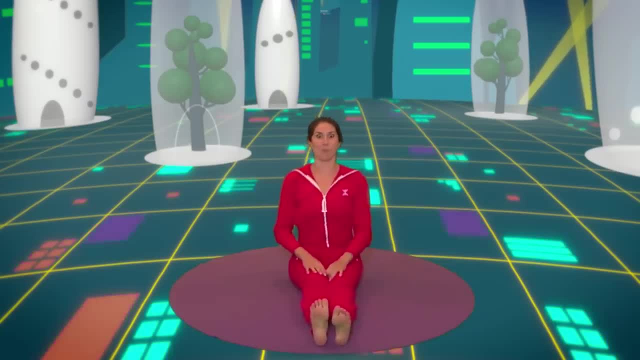 Mmm, Mmm, Mmm, Mmm, What's yummy strawberry yoghurt. Oh, I'm feeling quite full now, But then we hear the funny noise again. Shoo Sparks 24's tummy has turned from green to red. 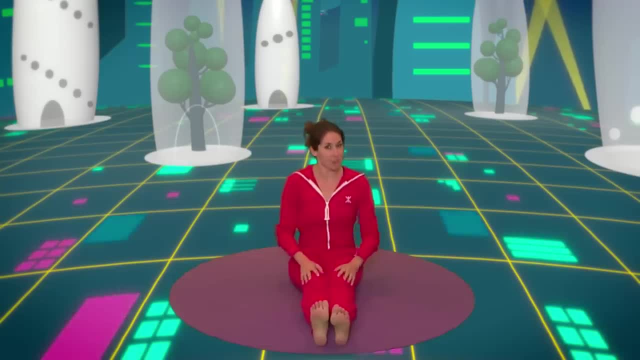 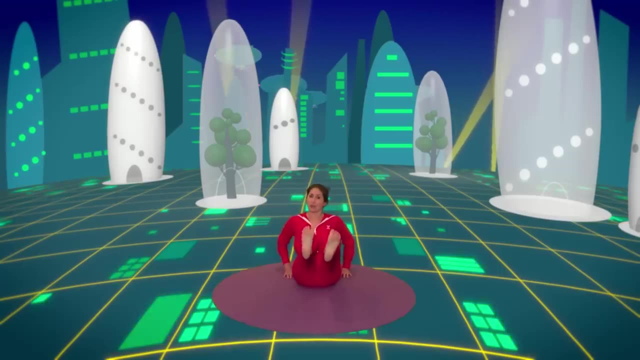 Oh no, Let's do the check. Is it his back paws Sitting back, Lift up your feet, E e, e, e, e, e e. No, they still work. Maybe it's his front paws. 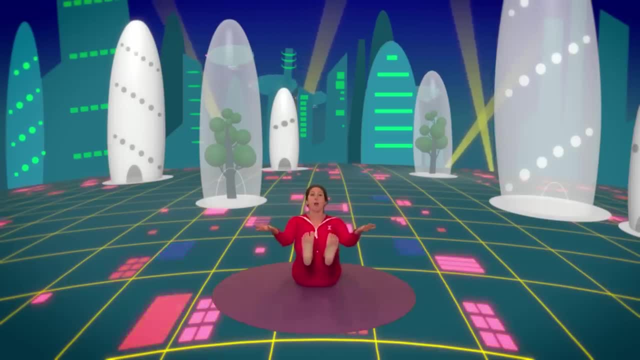 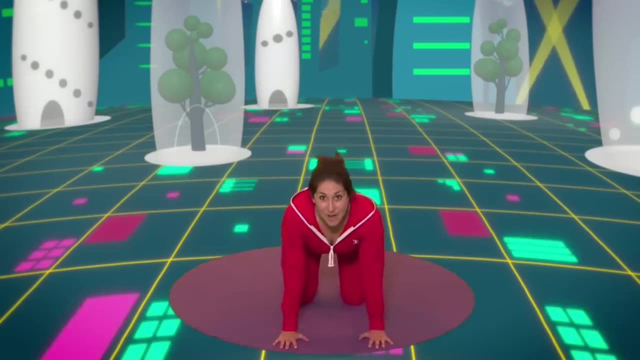 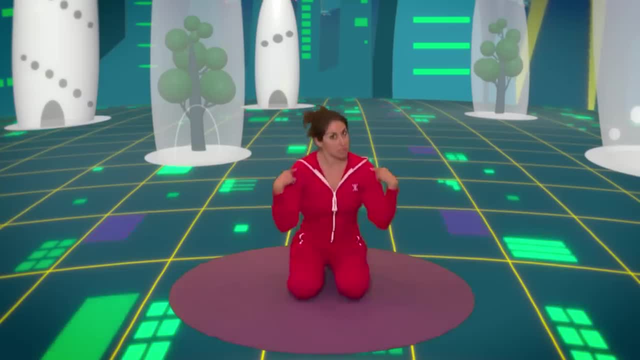 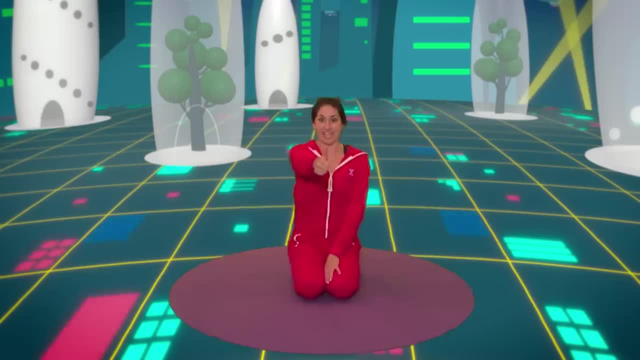 Maybe it's his eyes. Stick your thumb out. Let's see if we can follow that thumb with our eyes without moving our heads. Ready Up, Mmm Down, Mmm Side, Mmm Side. It's his eyes. 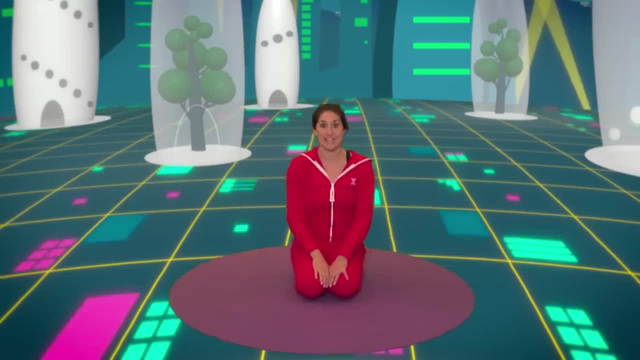 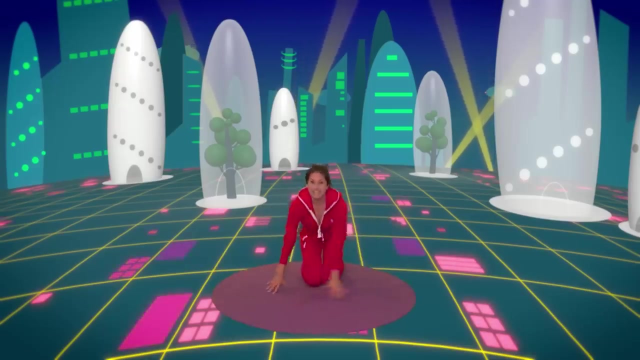 Let's switch them back on again by doing five slow blinks: Ready: One, two, three, four, five. Sparks 24 is here again. He does another big spin, Comes back down onto his back legs, stretches out his front legs and says: a happy robo dog, thank you. 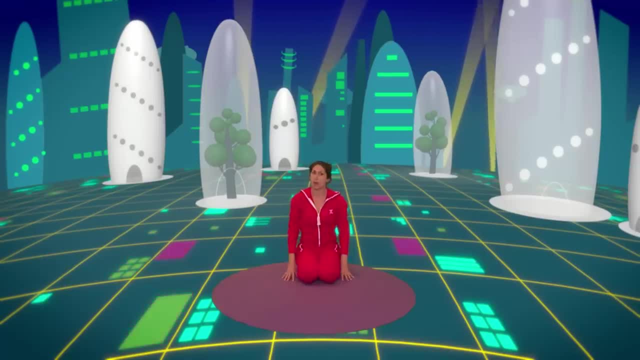 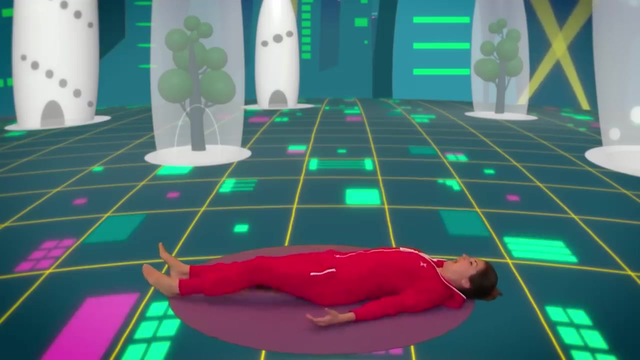 Sparks 24 thinks we should go to the relaxation pods now because we clearly need to recharge our batteries. What a lovely idea. We could do with recharging our batteries as well. So we head to the relaxation pods and plug ourselves in. We lie all the way back onto our backs and put our arms down by our sides. 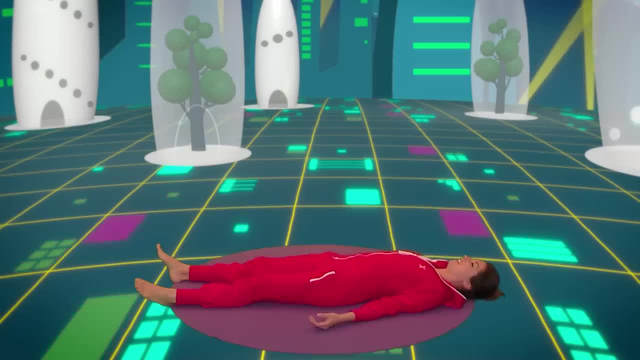 Ah, what a lovely thing to take a few moments and recharge our batteries. Sometimes bits of our bodies can switch themselves off, like our ears. We stop listening, And it's just good to notice when a bit of our body switches off, so that we can help it switch back on again. 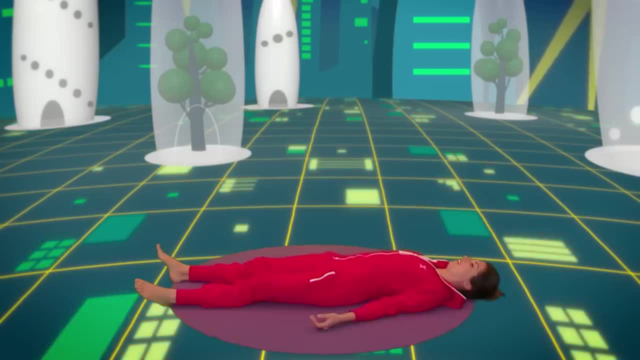 Just like we helped Sparks 24.. And now we can take this moment of peace and relaxation just to get our bodies feeling really good again. Let's take some lovely deep breaths, Very slowly. we start to wiggle our fingers and we wiggle our toes. 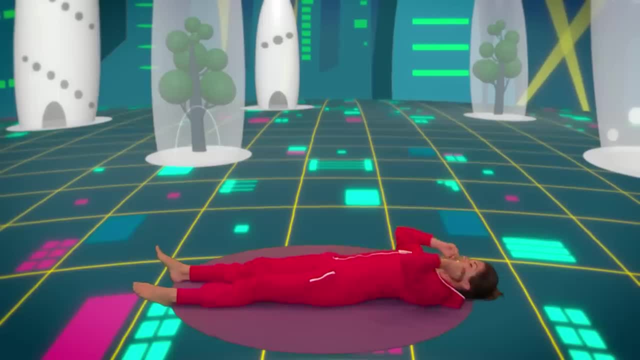 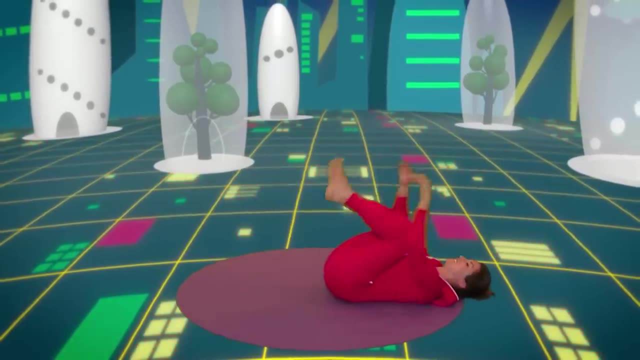 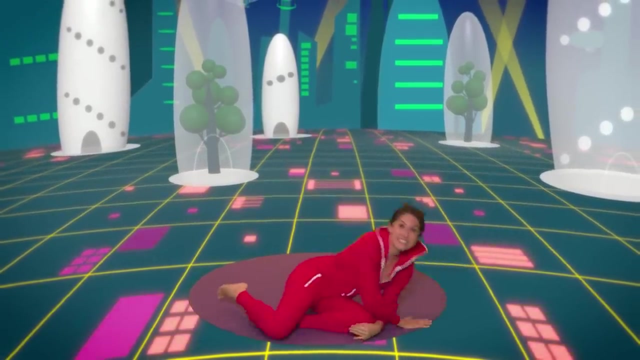 We stretch our body up really long like spaghetti. Then we bring our knees into our chests and give ourselves a cuddle. We roll over onto our sides and come up to sitting With our legs crossed, Just the way we started, with our hands together at our hearts. 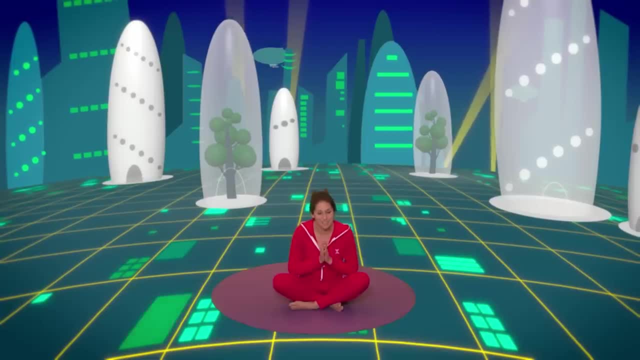 And we finish with our secret magic yoga code word, Which is: Namaste, Ready, One, two, three, Namaste. Well done everyone. Thanks for coming to the future with me, For meeting Sparks 24.. He loved you. I'll see you again soon for another Cosmic Kids adventure. 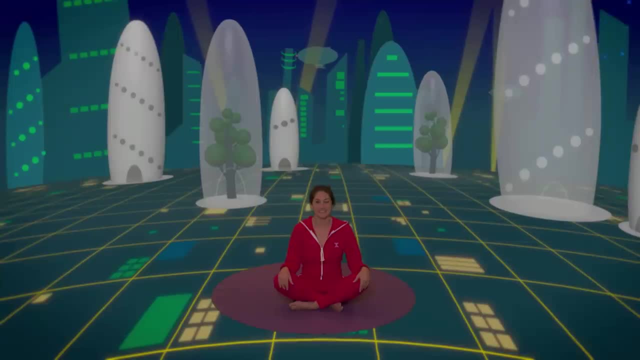 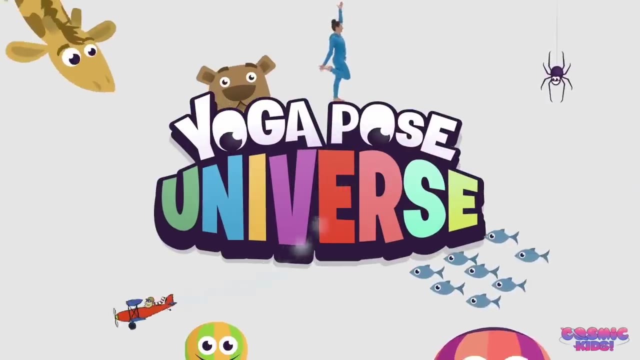 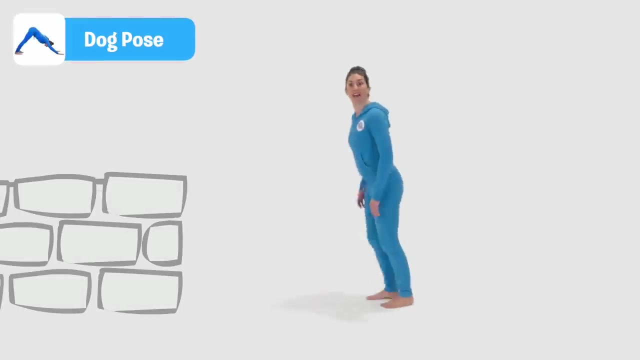 Bye, bye. The Cosmic Kids Yoga Pose, Universe Dog pose, Coming down onto our hands and our knees. We spread our fingers wide, Tuck our toes And press our hips up to the sky. Yes, Now look, There's a friend. 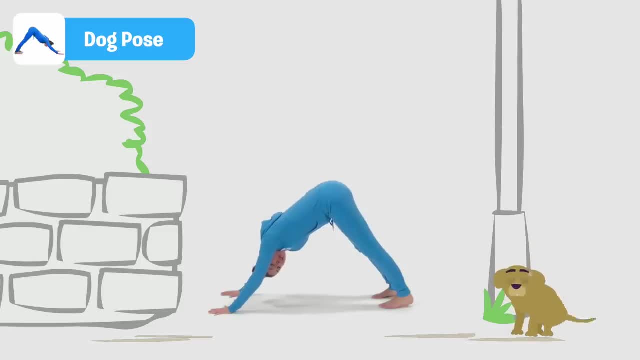 Hello. Aww, That's nice. Now, dogs always like to wag their tails when they're pleased to see you, So let's try that now. We reach up with one of our legs and we give it a wag. Waggle, waggle, waggle. 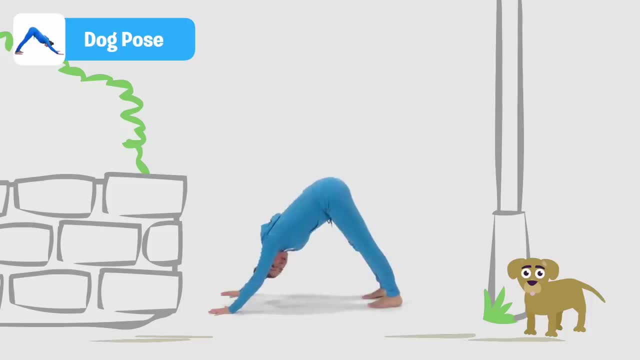 Very good. Lowering it back down Now dog pose is very good for strengthening our arms and stretching the backs of our legs, And because we're upside down, we get lots of lovely fresh oxygen to our minds, So it's very good when we're feeling a bit tired. 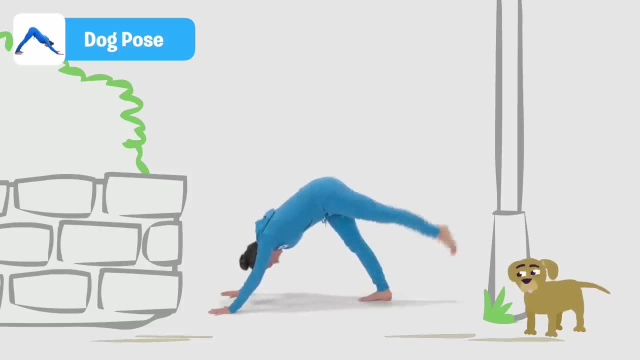 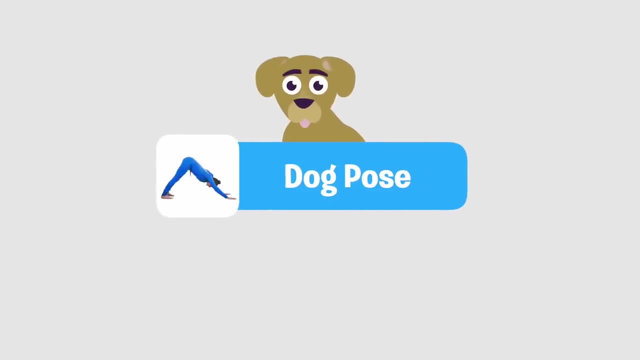 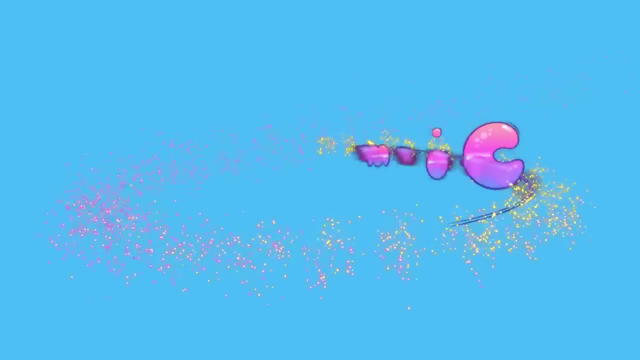 Let's try wagging our tail on the other side now, Stretching our other leg up and giving it a wag. Waggle, waggle, waggle. Oh, thank you, I love you too. Dog pose- Hello everyone. Welcome to Cosmic Kids. 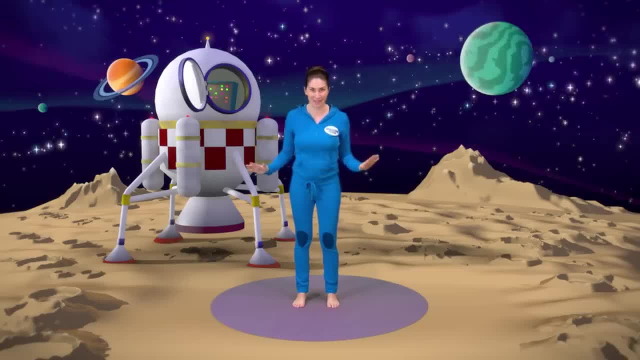 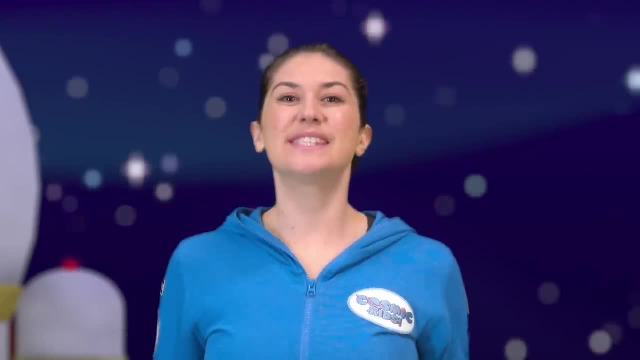 I'm Jamie, and this is your place for yoga stories and fun. It's easy: Just copy the moves I do and enjoy the adventure. Now, we always start in the same way, And that's by sitting on our bottoms, Crossing our legs. 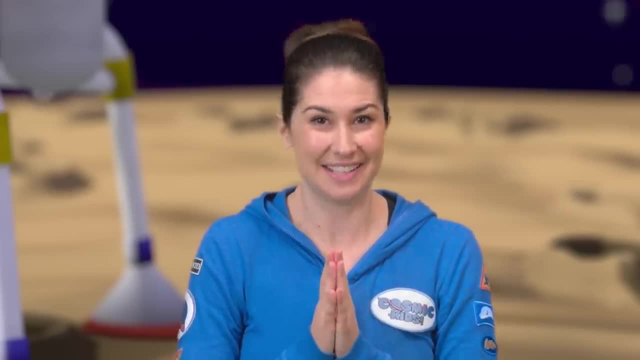 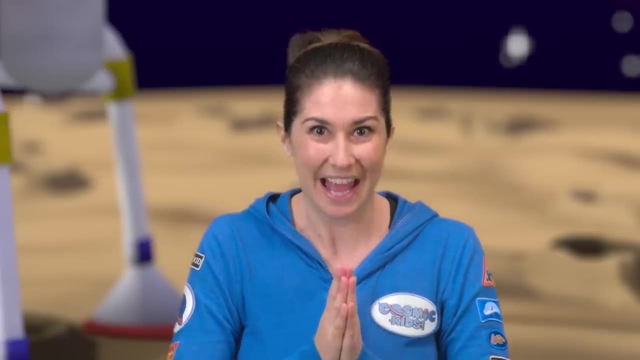 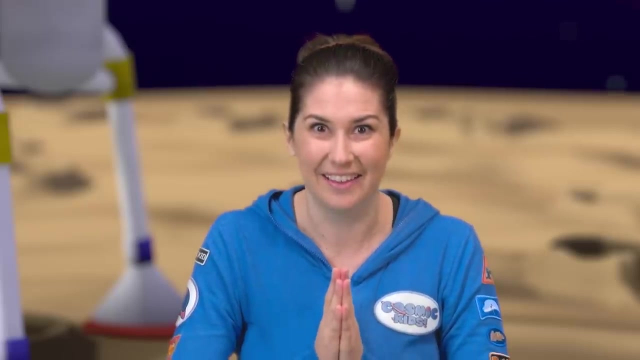 And bringing our hands together at our hearts And saying our secret yoga code word, Which is Namaste, Ready After three. One, Two, Three, Namaste There. Now let's have a look through our cosmonoculars and find out who we're meeting today. 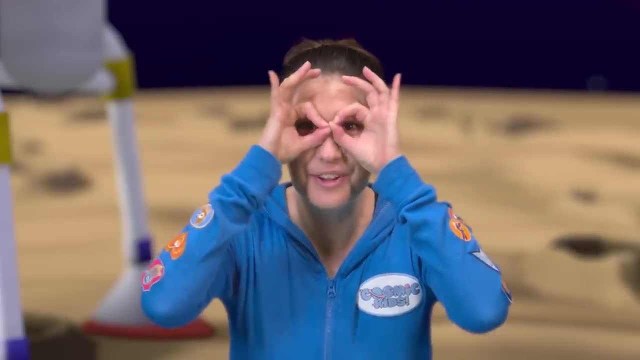 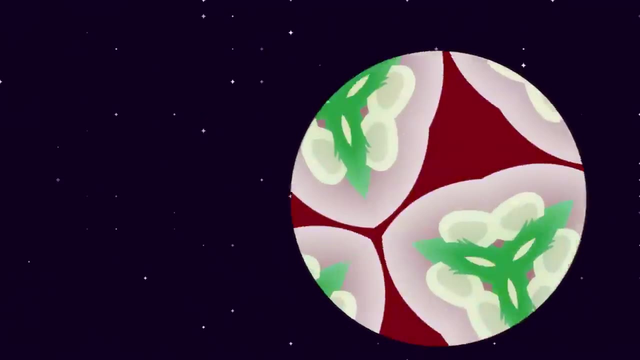 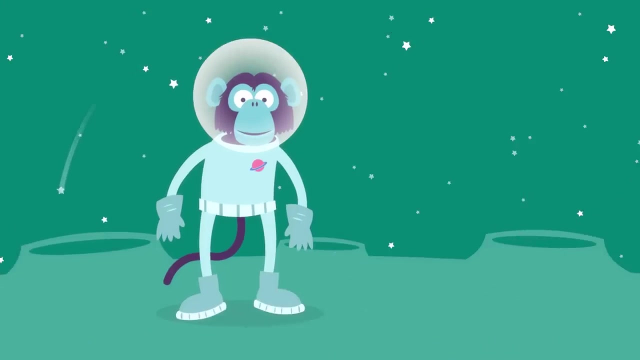 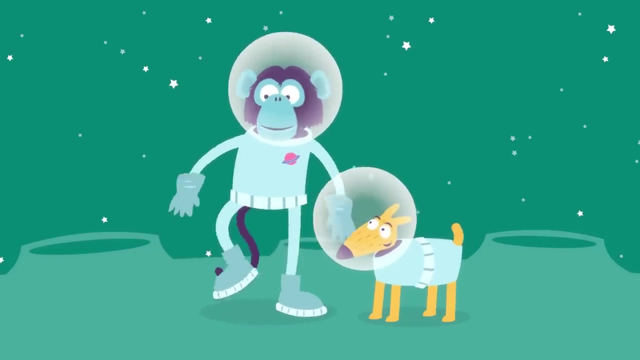 Joining your thumbs and fingers together. Have a look through. Oh, look at the colours all spinning around. They're amazing. Oh, look the shapes. Can you see the picture? Yes, Look, It's a monkey and a dog. It's Mike, the Cosmic Space Monkey. 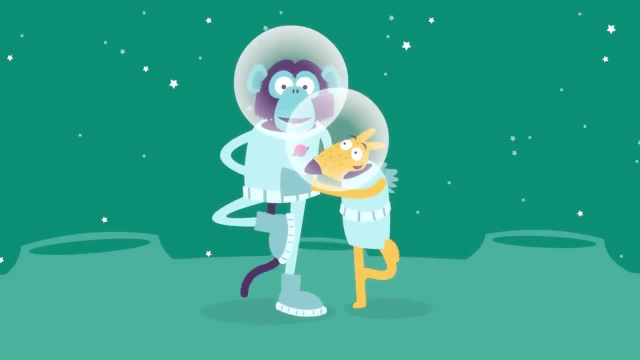 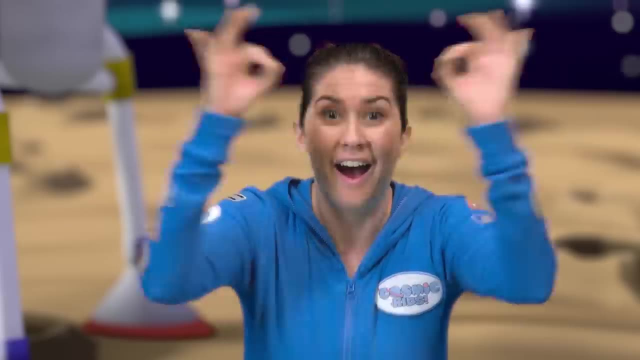 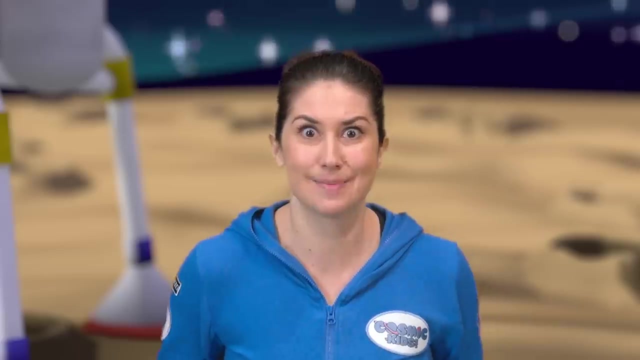 And Mutnick the Astro Dog. What are Mike and Mutnick doing? They're doing yoga. They're doing double tree pose. This is so exciting, Mike and Mutnick. they live on the moon, So that means we're going into space. 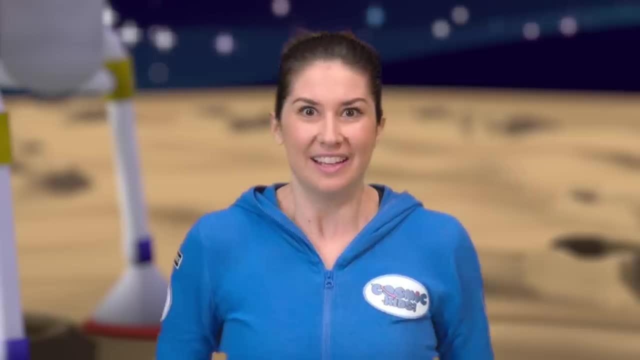 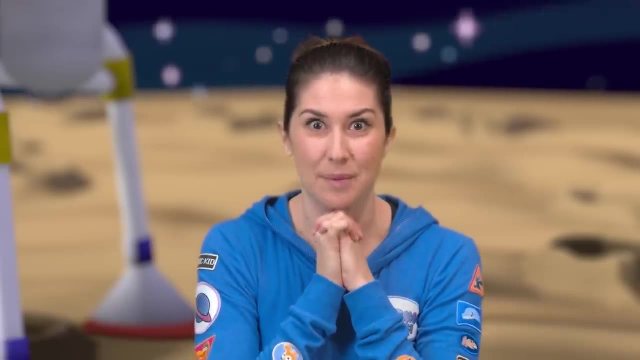 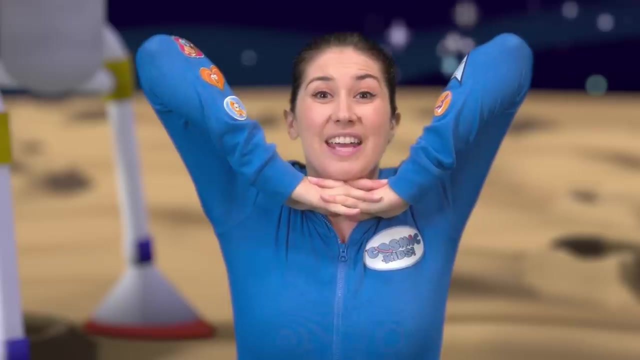 We're going to the moon. This is so much fun. Let's start by taking some big, brave breaths. We criss-cross our fingers and put them under our chin And we take a big breath all the way in, Ready, Lifting your elbows high, high, high. 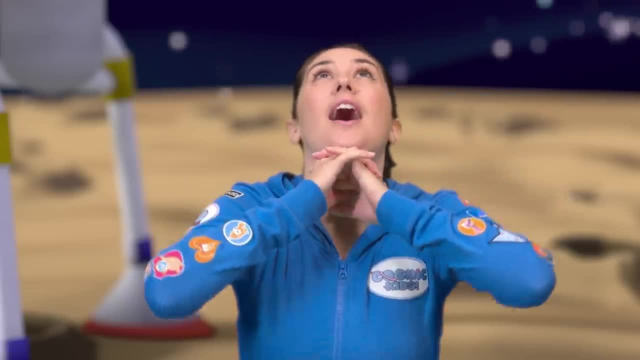 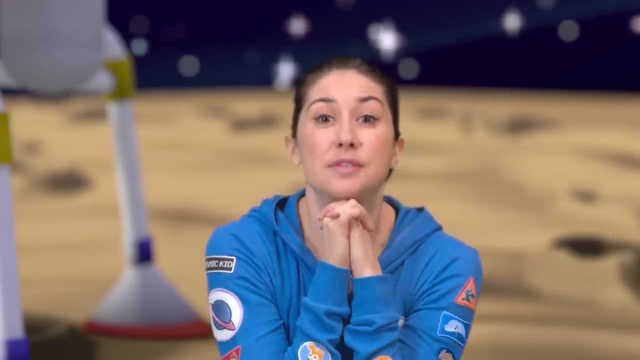 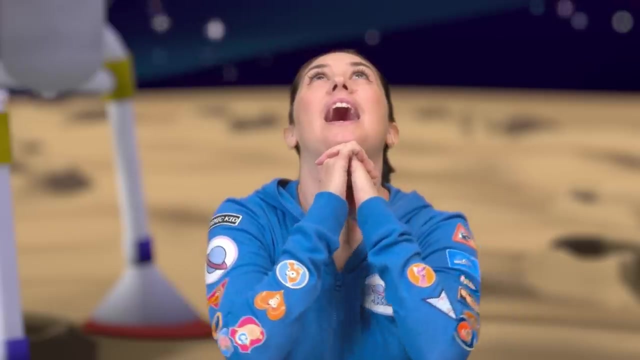 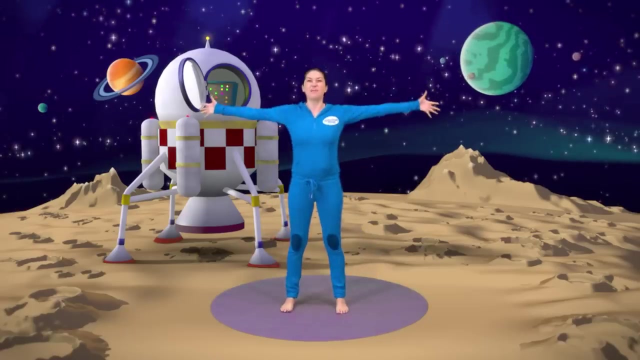 And then we breathe up to the sky. Ready, Let's do another one of them: Breathing in, lifting your elbows, And breathing out to the sky like a dragon. Very good, everyone, Let's stand up now and take our arms wide. 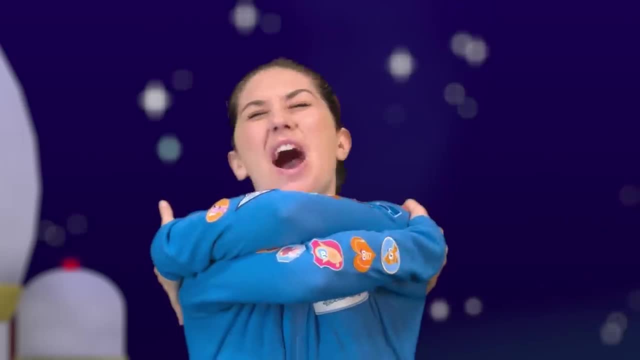 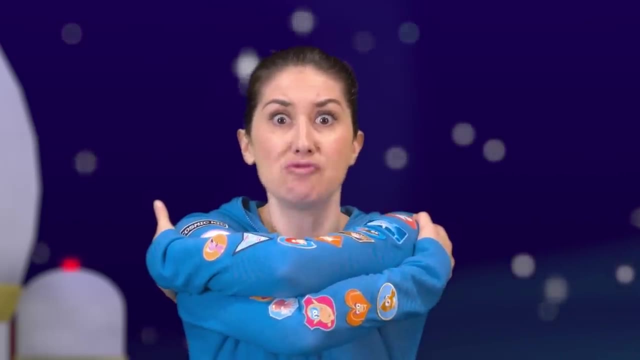 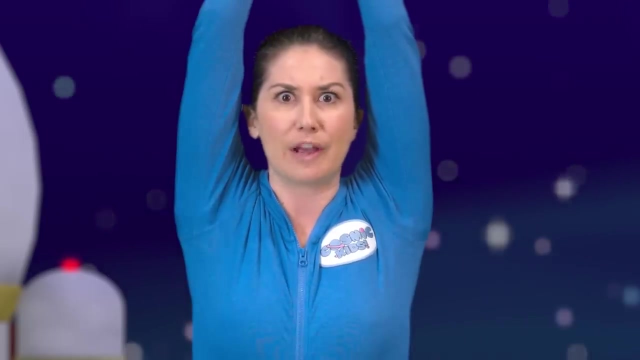 to give everyone at home a great big hug. goodbye, Bye, everybody. And out of the corner of our eye we spot outside in the garden, our rocket. Jump your feet wide, take your arms wide and bring your hands above your head. Look at our rocket, everybody. 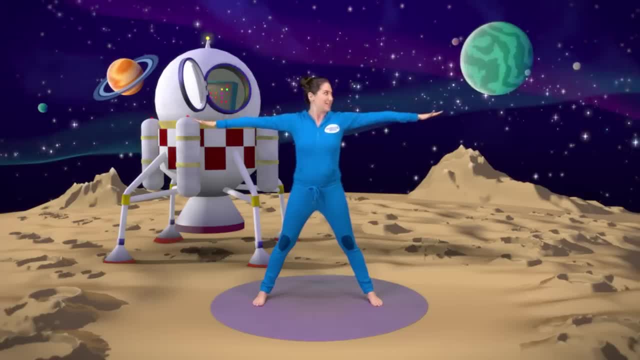 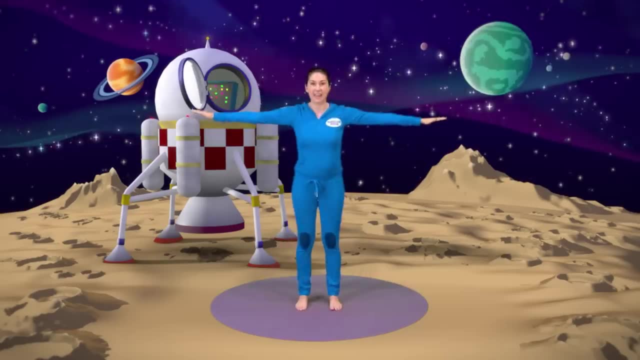 And look, take your arms out to the side. It's got great big giant silver wings. Cool, Let's go and get in. We jump our feet together, We squat all the way down And then we sit with our legs out long. 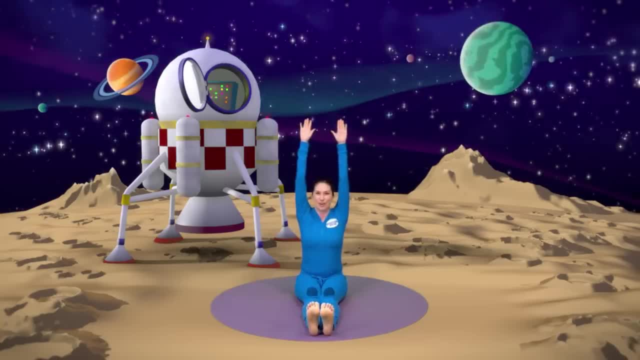 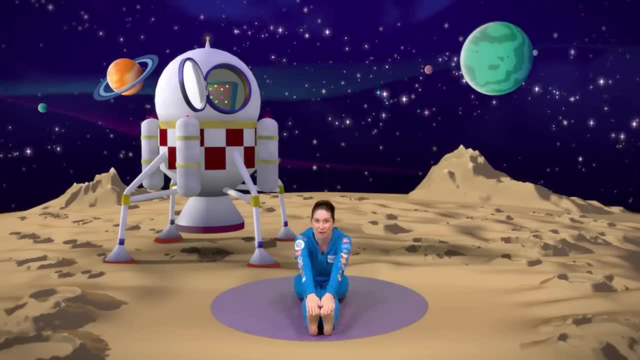 We reach up and we close the big glass door on our rocket, Bending our knees a little bit to touch our toes. Now we're in our rocket. we activate our ears by giving them a rub all the way round so that we can hear important messages. 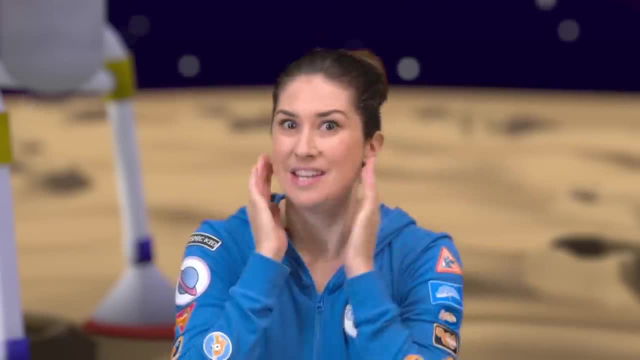 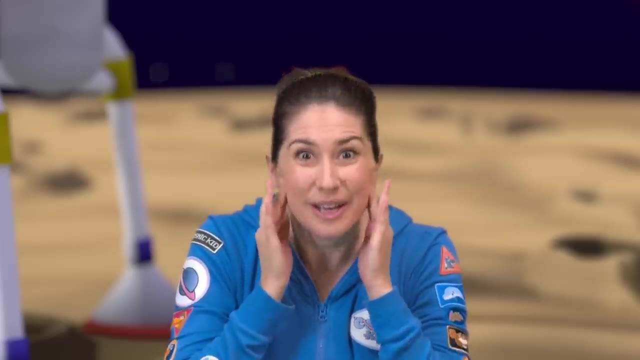 Oh, and we need to activate our voices So we give our jaws a really good rub as well. Well done everyone. That means we can speak too. Now we need to turn our rocket on, So we fold forwards and we turn on all of the knobs and beepers. 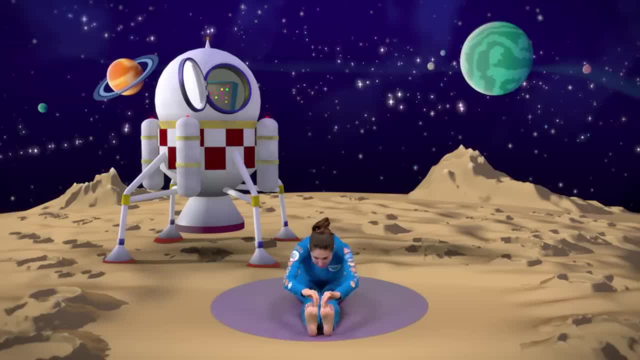 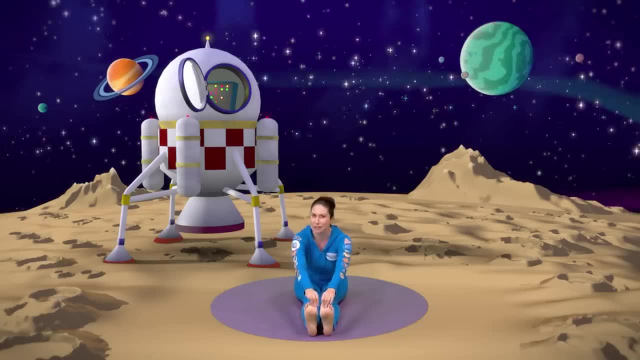 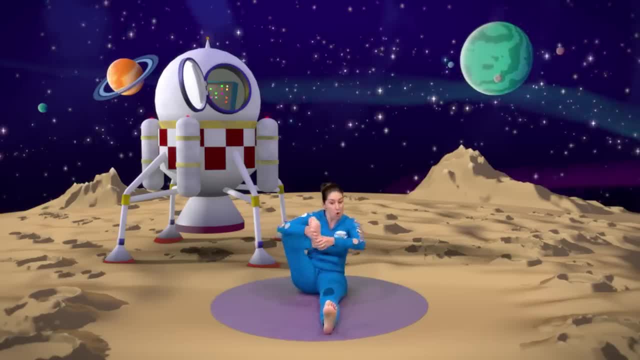 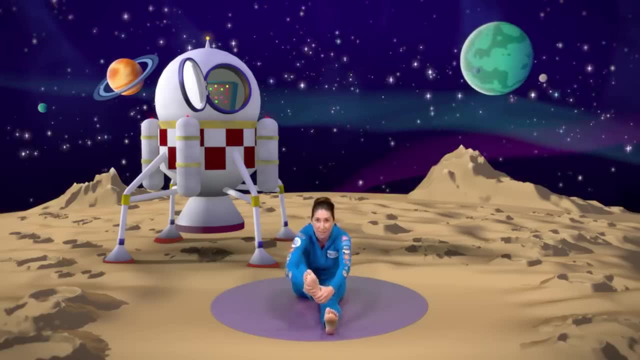 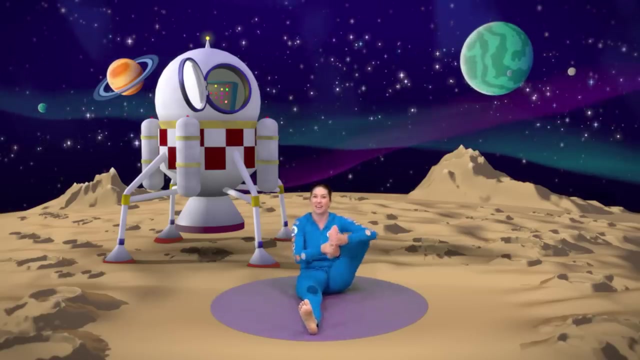 Lift up one of your feet and take it over one side And the other, All the way forwards And all the way back. Well, that one works, Let's try the other. Putting that one down, Lifting up the other side now. 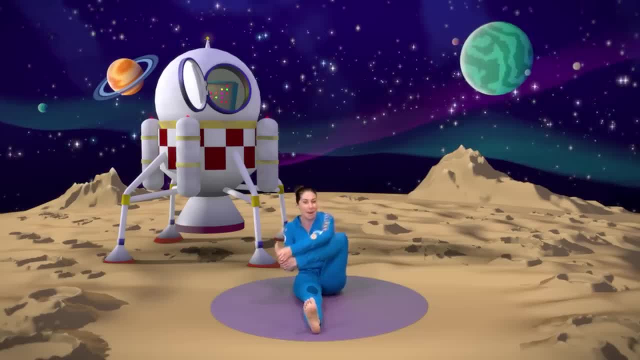 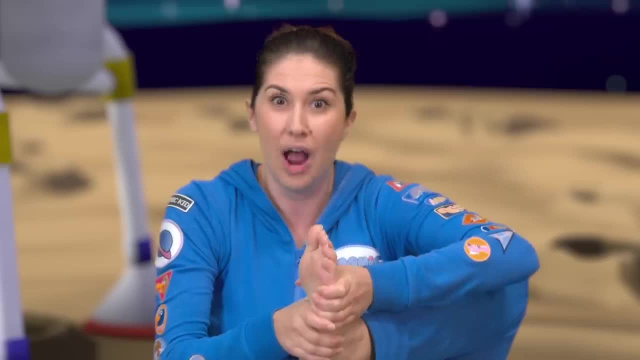 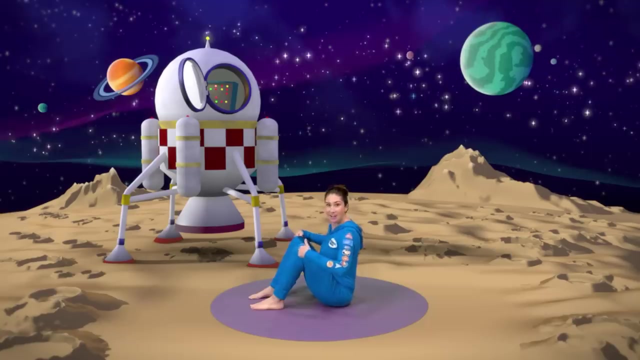 Ready And the other way, Forwards And backwards. That one works too. I think we are ready for take off Now. turning to the side, We bend our knees, Put our feet flat and take our hands behind us, And as we lift our hips, we count down from five. 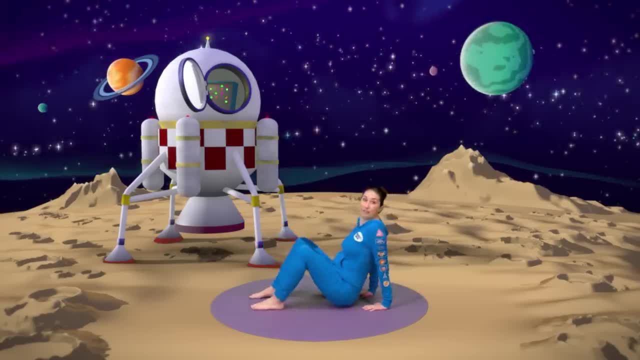 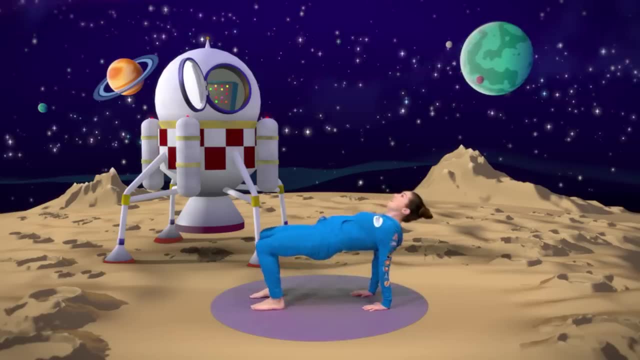 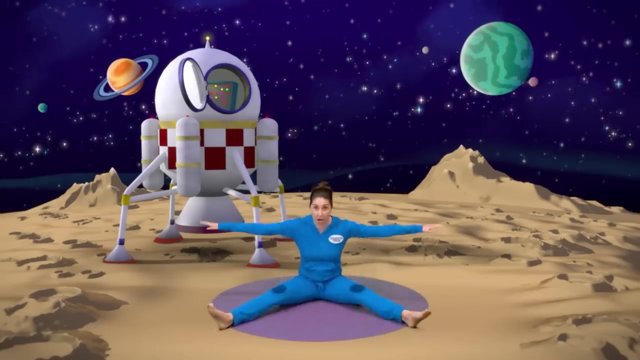 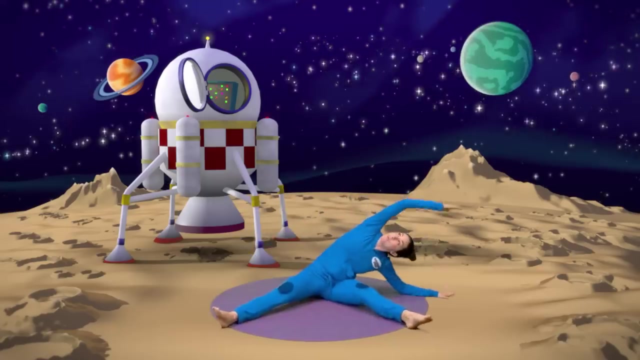 Ready? Here we go, Five, Four, Three, Two, One And blast off. We sit with our legs wide, everyone, As we rumble up into the sky. We go over to one way And over to the other way. 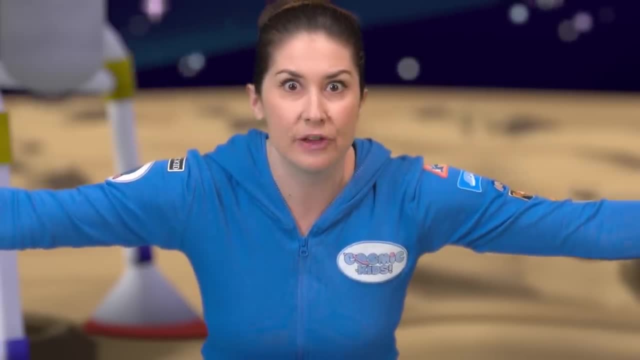 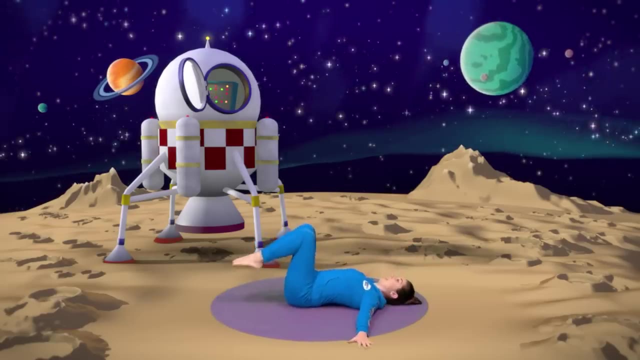 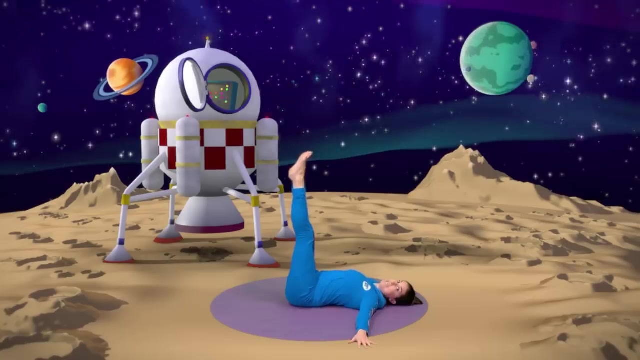 And then we break through Earth's atmosphere And we feel zero gravity. We lie on our backs In our seats with our arms wide And our legs float all the way up. Wow, We're going into space And it's so lovely. 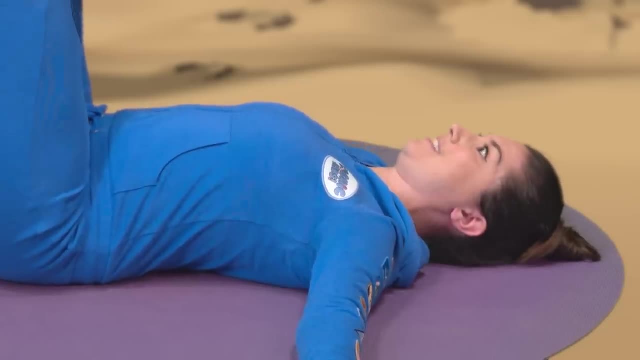 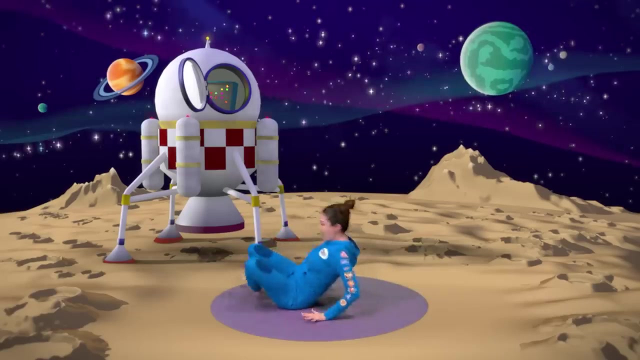 Outside our window We can see a gazillion stars. It's so peaceful out here, Amazing. Did you hear that? Yes, It's the landing warning. We need to get into our landing position, Coming up everybody Onto your knees. 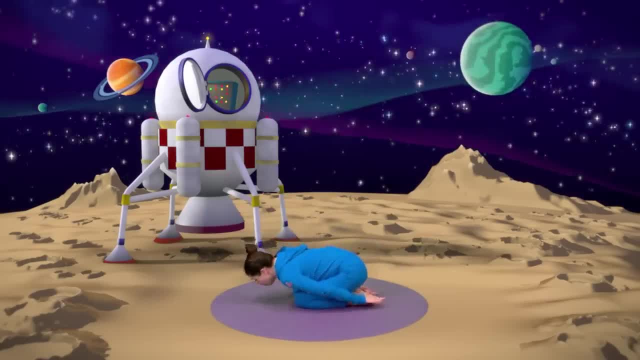 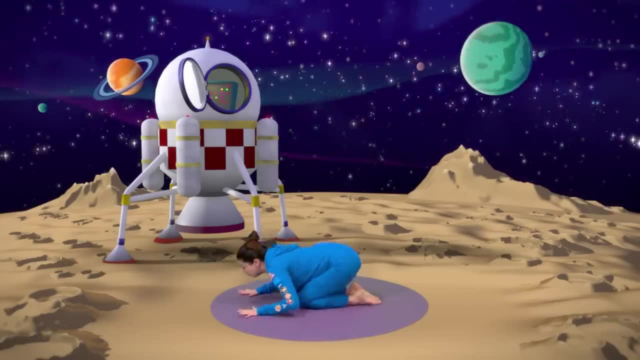 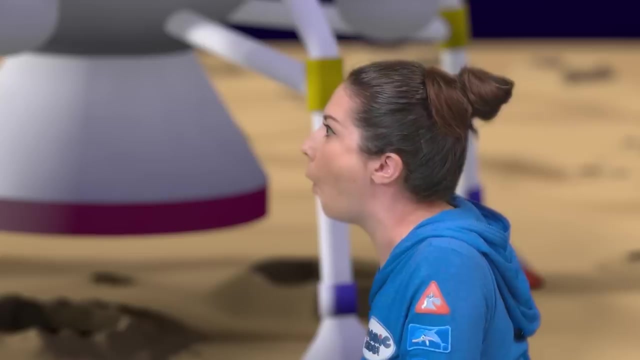 Tuck yourself up into a tiny little landing ball. We've landed on the moon. Let's wiggle forwards onto our bellies And have a look through our little round window. Wiggle, wiggle, wiggle. Oh, Look out there everybody. 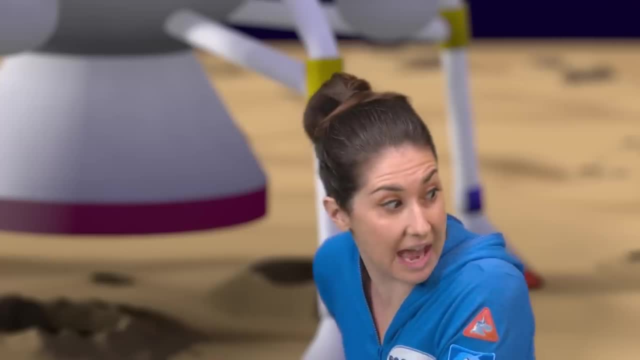 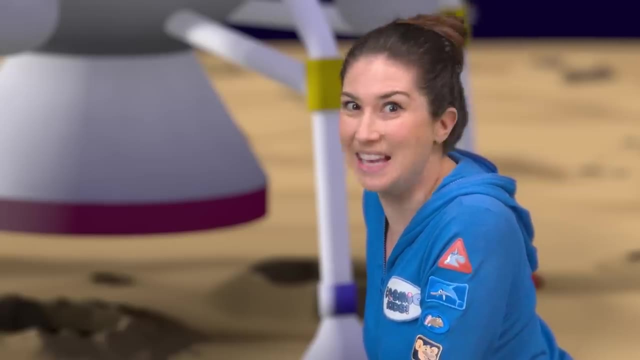 It's the moon. We check our wings are okay. Looking to each side, Yep, And looking forward, We can see Mike, The cosmic space monkey. Let's get into our space suits, Coming up to stand everyone. We stand up tall. 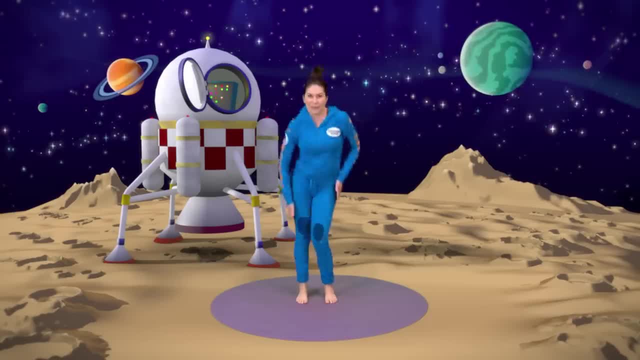 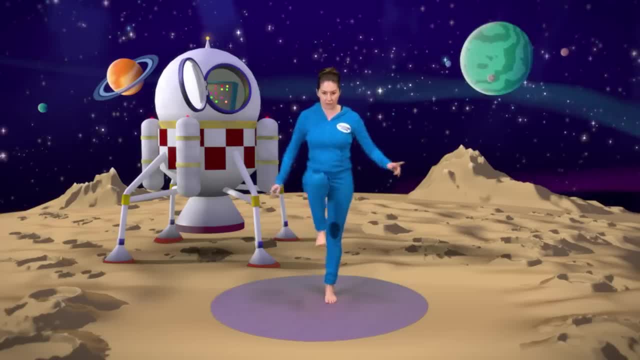 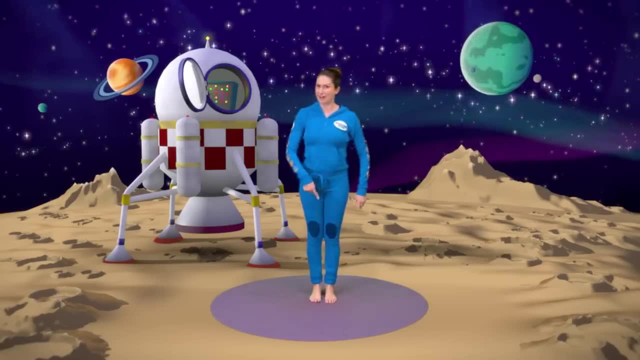 Now we need to put on our jet pack moon boots. We lift up one foot- Oh, try not to wobble- And we put our boot onto our foot. Very good, everyone, Let's try the other side now, Lifting up the other foot. 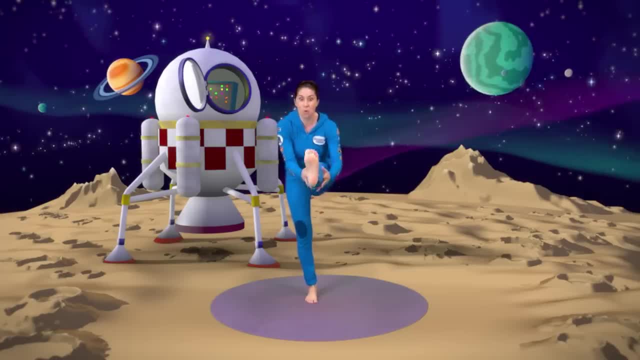 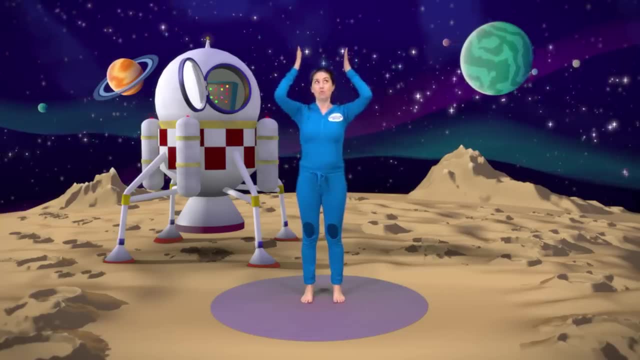 Holding onto our moon boot And pop it on. Very good. Now our helmets. We reach up for our helmets And we put it on our head, Making sure it's secure at the neck And all of our oxygen works Very good. 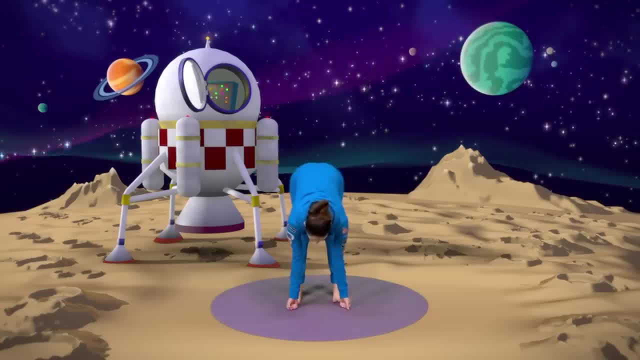 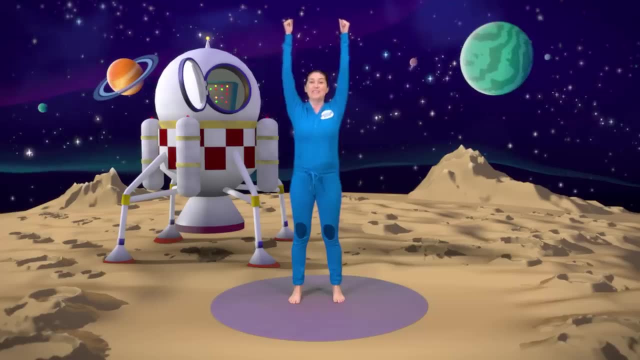 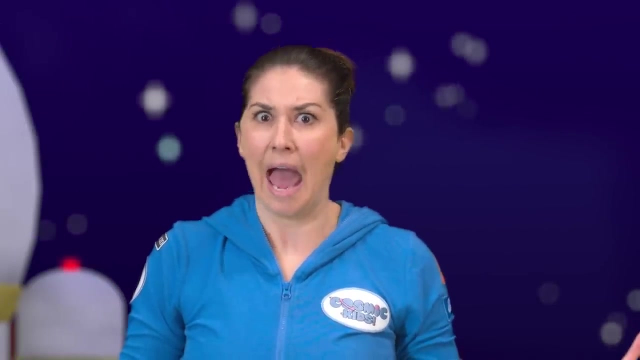 Now we need to open up the door. We reach forwards And we lift it up, Opening the big glass door. We say hello space, Hello space, And Mike, the cosmic space monkey, is here And he does a big anti-gravity monkey jump. 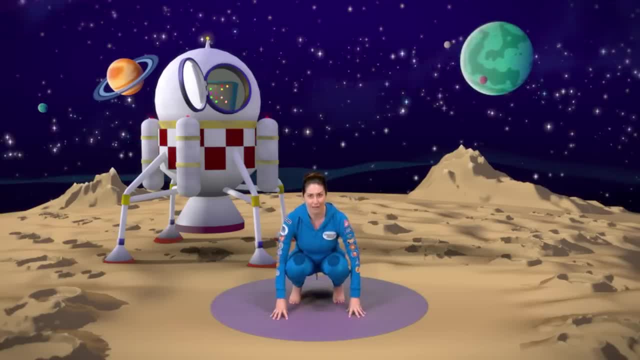 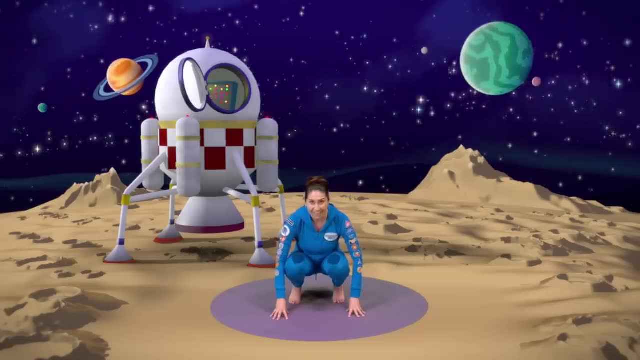 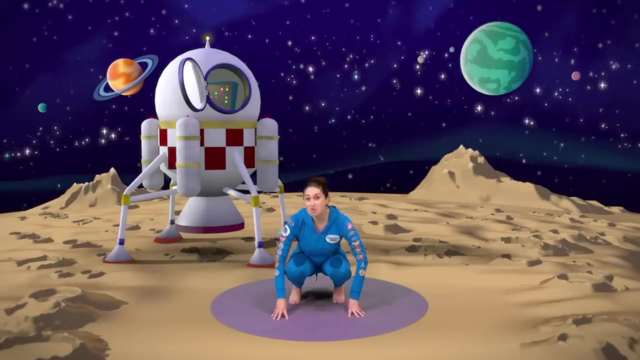 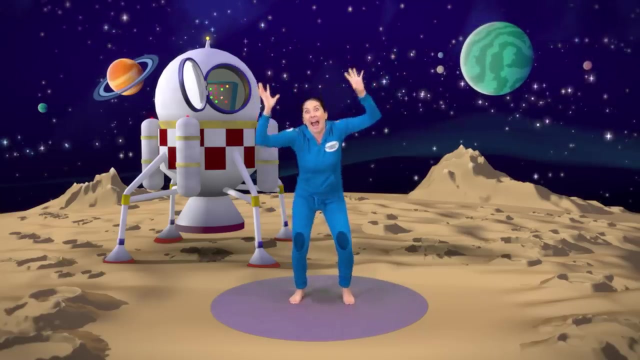 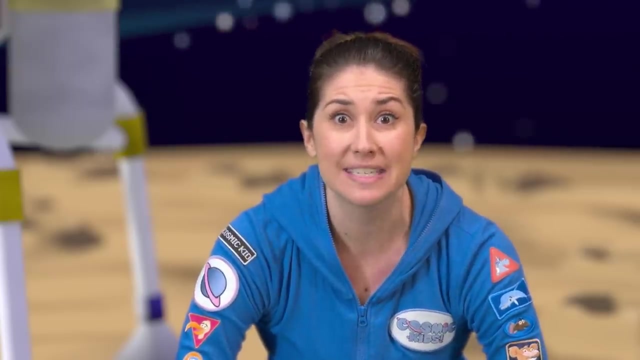 Now coming down to crouch. It's quite hard doing a monkey jump in anti-gravity Because it happens very, very slowly. Ready After three, One, Two, Three, One. Oh, Mike, the cosmic space monkey. Oh, I'm so pleased to see you. 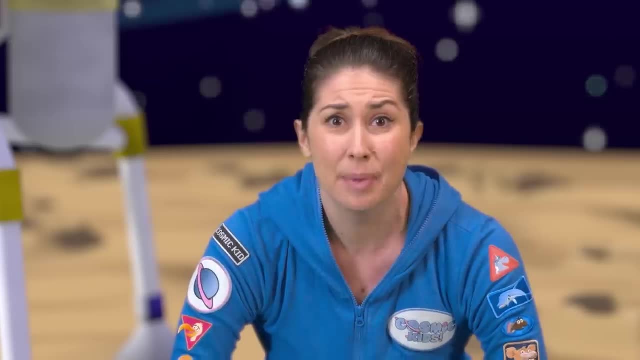 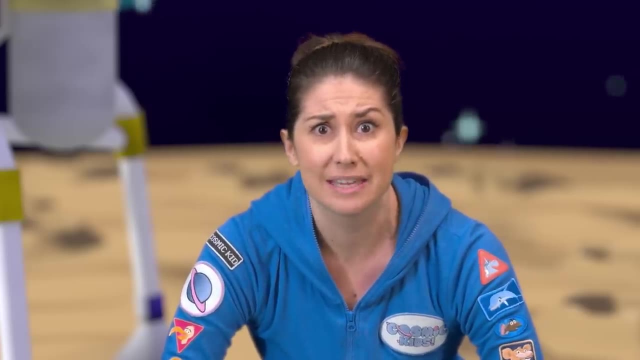 It's great that you've come all this way. You're such good friends, But I need your help. My astro dog Muttnick- He's my best friend. He seems to have disappeared. I can't find him. Last time I saw him was this morning at the Milky Way cafe. 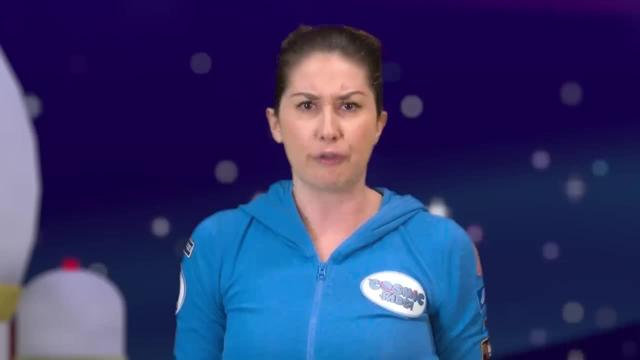 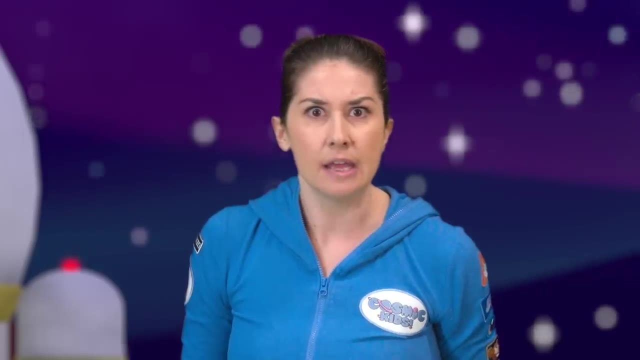 Do you think you can help me? We stand up. Well, good friends always do look out for each other. I think we can help Mike find Muttnick. Hey, Did you see that In the moon dust Look Folding all the way forwards. 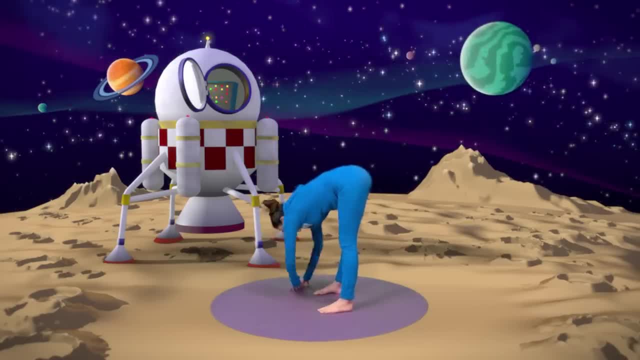 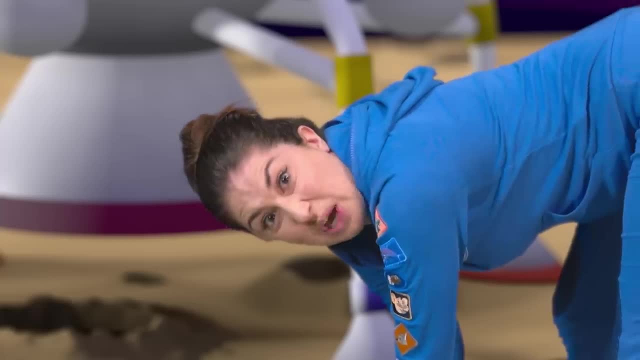 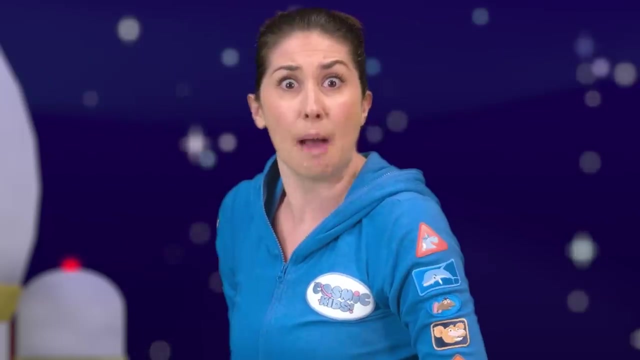 We can see something. Use your fingers to clear the moon dust. It's a footprint of a cybersaur. That's a space dinosaur. And stand up everyone, because we can hear it coming this way, Turning to the front Legs wide. 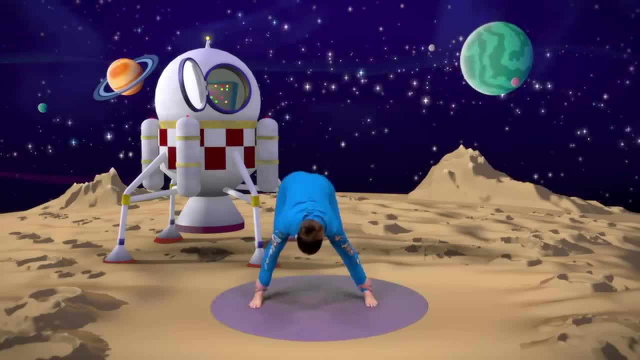 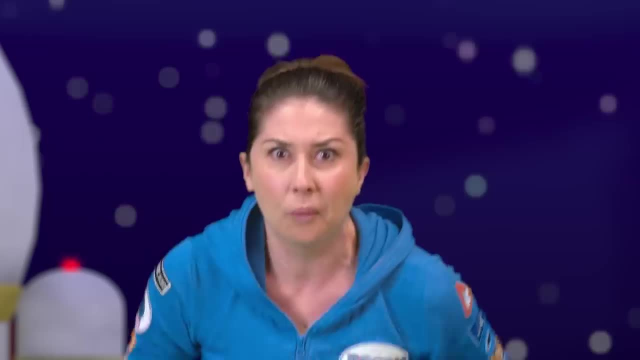 Fold forwards and hold on to your ankles. He's clumping this way: Clump, clump, clump, clump, clump, clump, clump, Quick everyone. We need to hide behind the moon rock And so he won't see us. 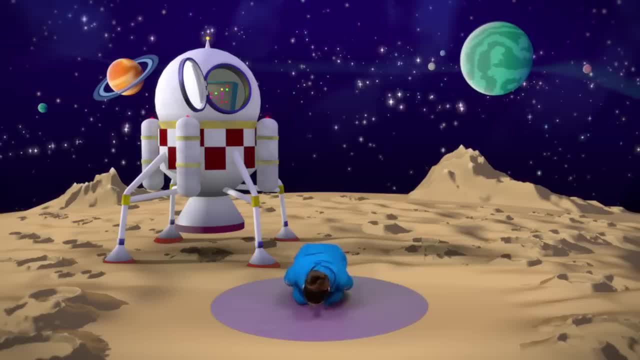 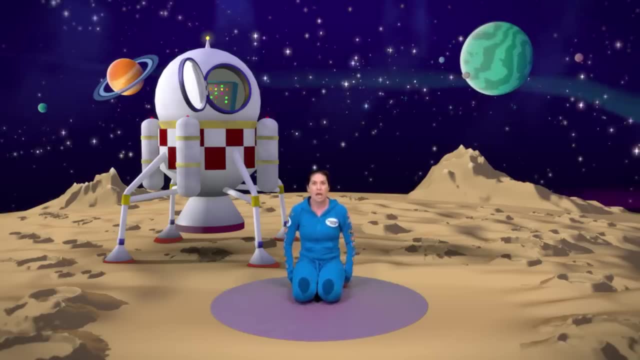 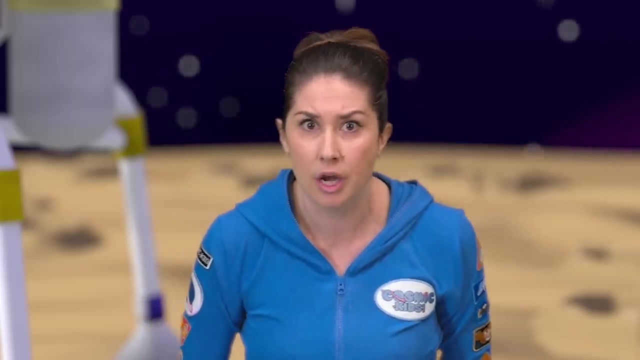 Tuck yourself down into a tiny little moon rock shape, Shh. We sit up after he's gone past And we say, Phew Gosh, that's a relief, We're glad he's gone. Maybe Mutnick was running away from the cybersaur and he got a bit lost. 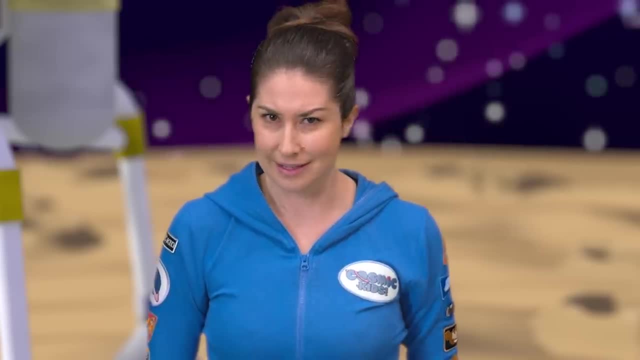 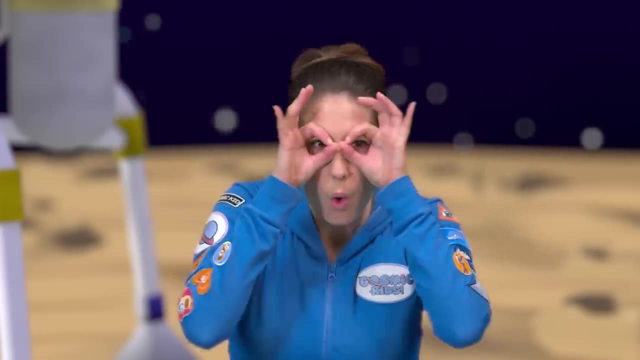 Hmm, Let's look through our cosmonoculars again and see if we can find him Joining your thumbs and fingers together. Have a look through. Oh well, it's quite hard to see anything because right in front of us. 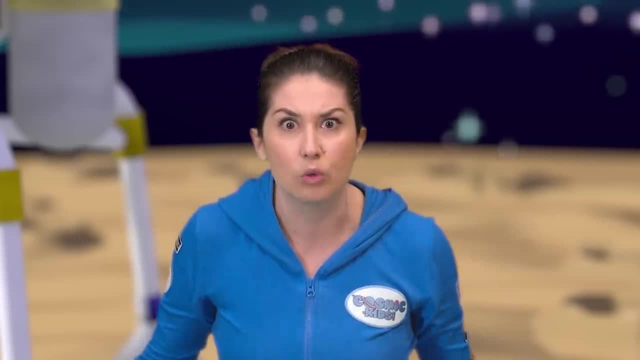 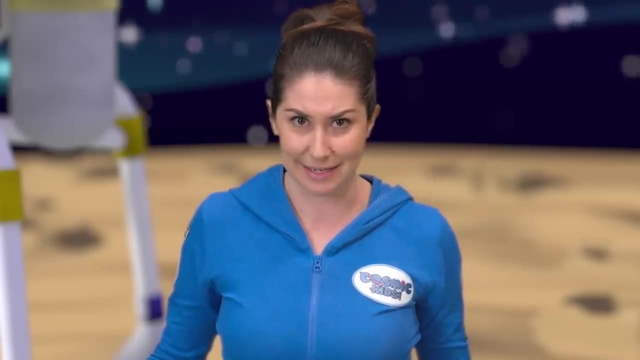 we seem to be looking at the sea of clouds. Oh goodness me, It's quite hard to see where you're going in the sea of clouds. For this we need a crater skater Coming up to stand everyone. We get on board our crater skater so we can be sonic surfers. 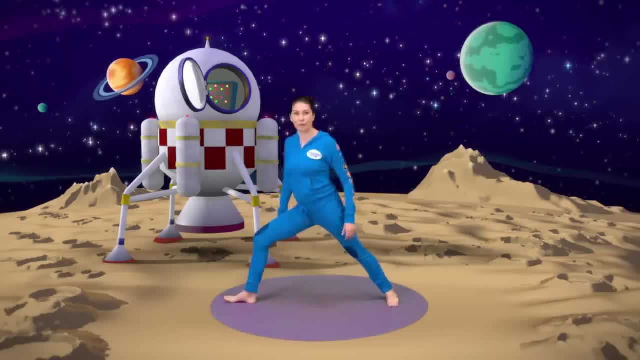 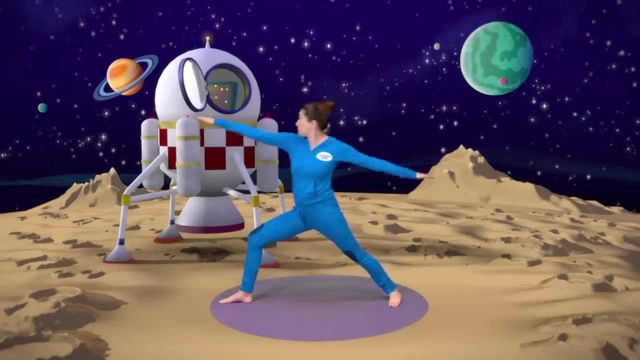 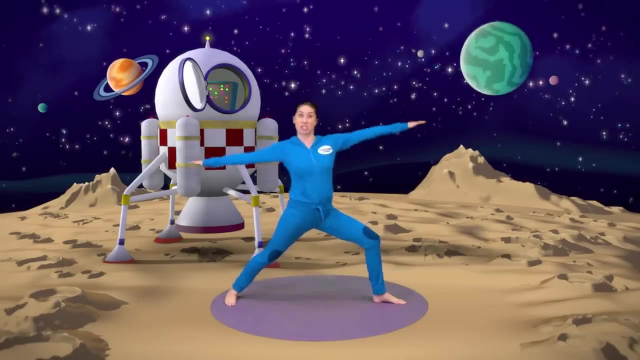 Put one foot forwards, one foot backwards, Bend your front knee, Take your arms wide And off we go, whooshing across the surface of the moon. Whoosh, We jump and do it the other way. Whoosh, Uh-oh. 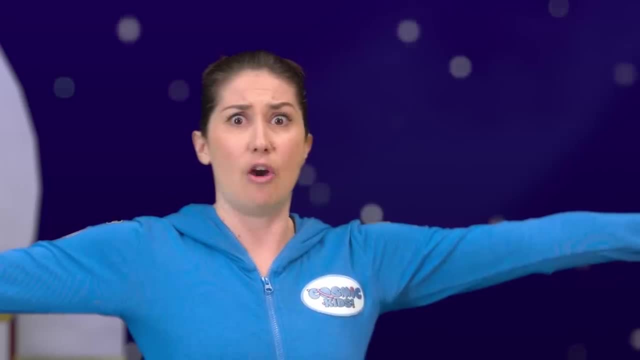 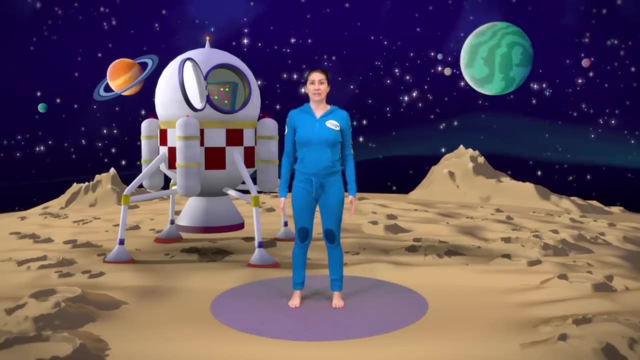 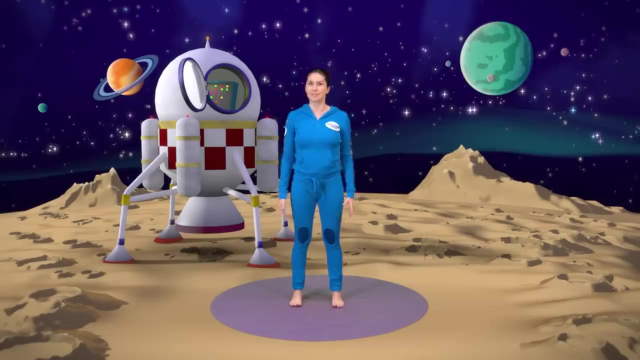 We've stopped. We've stopped because we're right in the middle of the sea of clouds and we can't see where we're going. So we stand with Mike like mountains, as still and as powerful as can be, Trying to listen with our special listening ears. 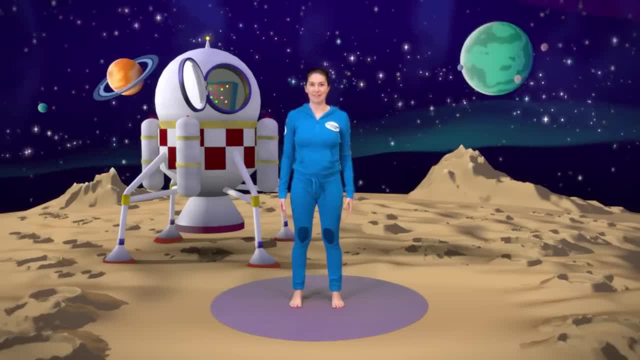 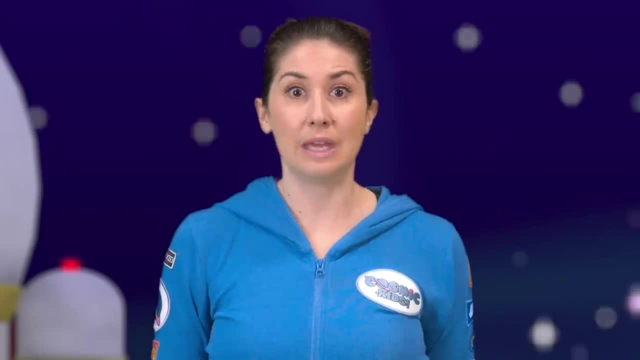 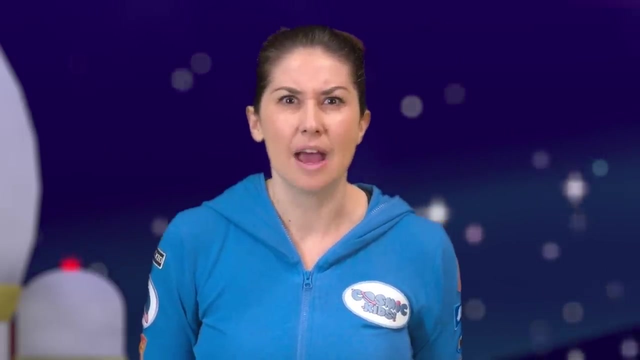 Taking your arms down by your sides and stand very still like a mountain. We hear something: Oowee, Oowee. What's that? Looking with our eyes, we can see through the clouds- A mermaid, Oh, but maybe it's not a mermaid. 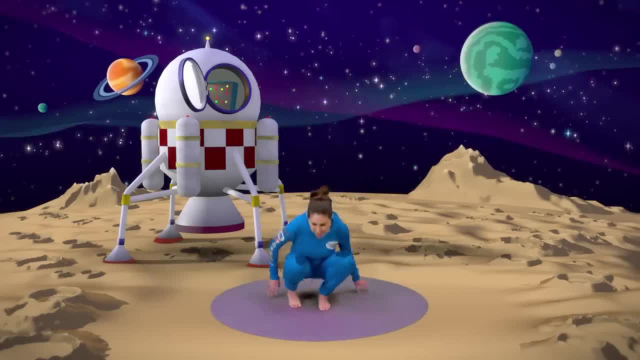 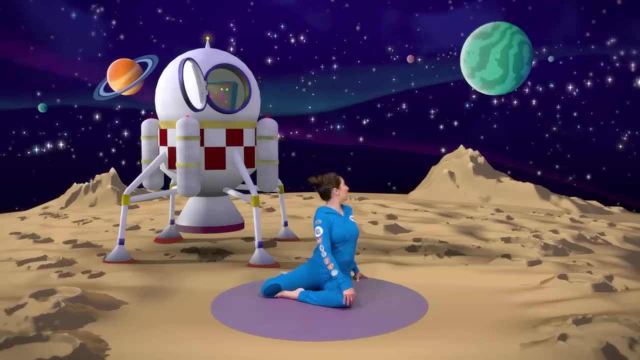 Maybe it's a moon maid sitting on your bottoms. Take your legs around to one side, Put one hand on your knee and the other hand behind you, Looking over your shoulder, then looking to the front. She says it again: Oowee. 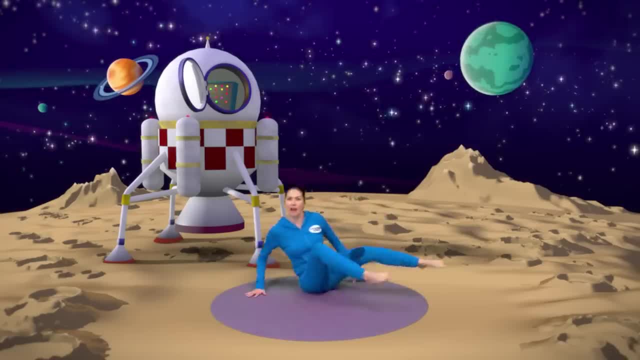 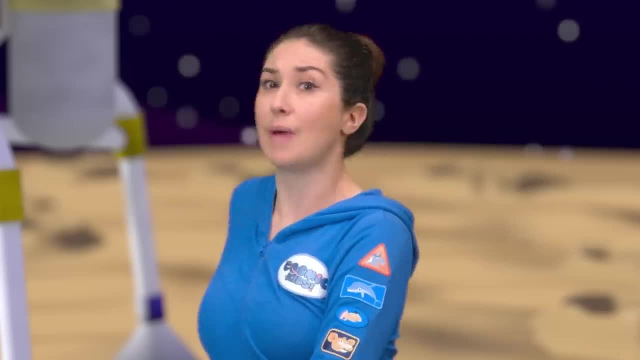 Oowee. Then she seems to swish her tail around to the other side. She puts her other hand on her knee, Her other hand behind her, She looks over her shoulder, She looks back at us and she says Oowee. 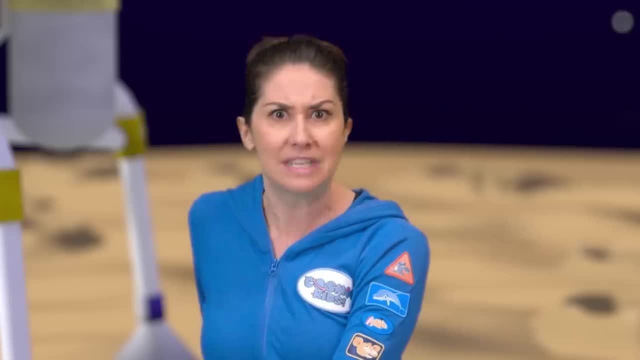 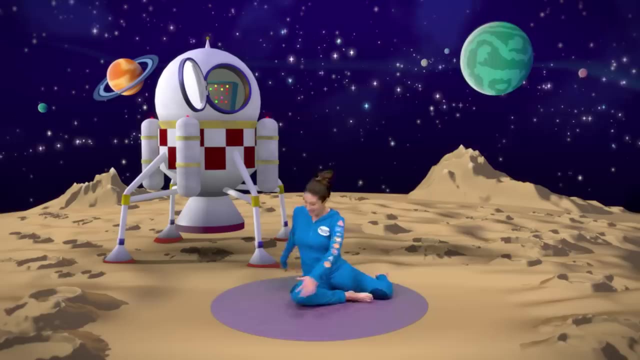 Oowee, She's calling us over. We better go and find her Now. to get through the sea of clouds, best thing is to go on our hands and knees so that we can see where we're going. Coming onto your hands and knees, everybody. 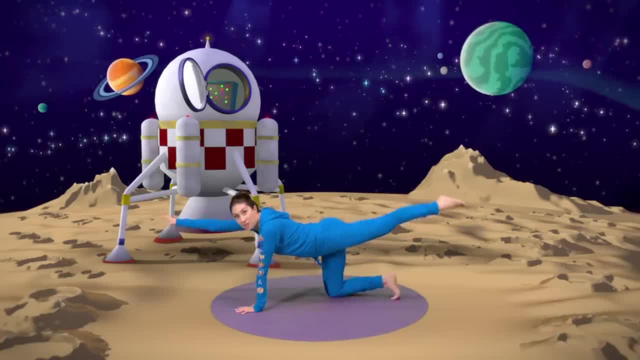 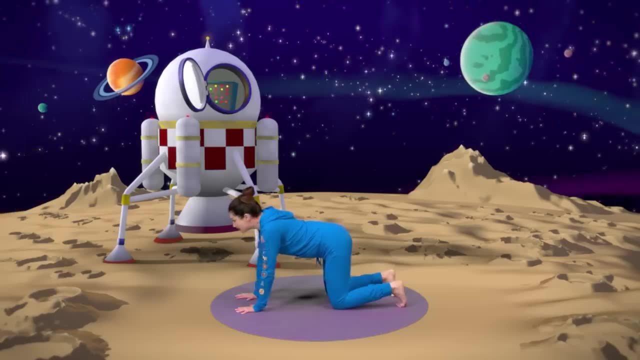 We reach forwards with one arm and reach back with the opposite leg. Oh, well done everyone. We bring that hand and that knee back down and we try it on the other side. Reach with one arm and reach with your opposite leg. Very good. 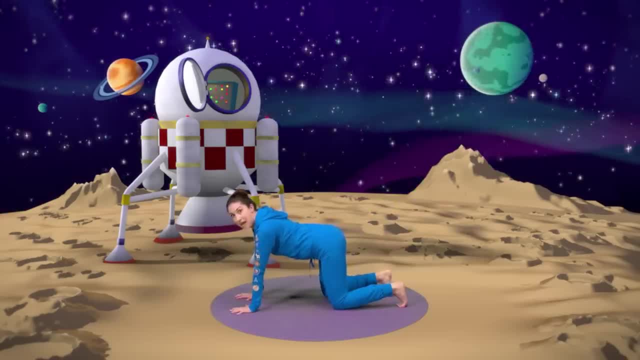 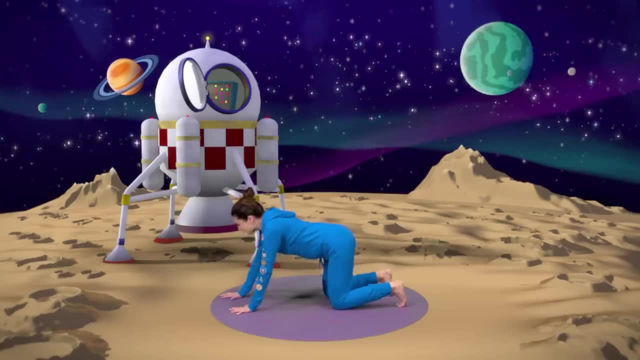 Strong tummies everyone And bring your hand and your knee back down. We make it over to the moon maid And sat next to her is Matt Nick, the Astro Dog. Hands forward, tuck your toes and lift your bottoms up. 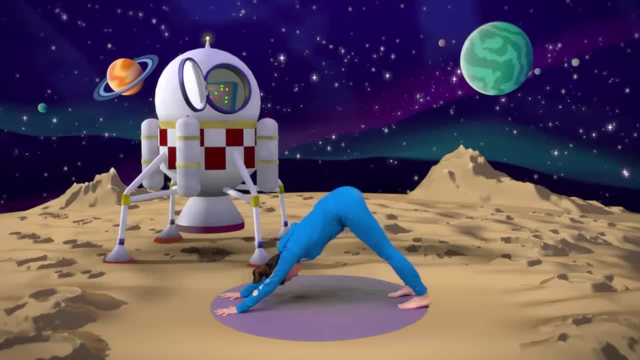 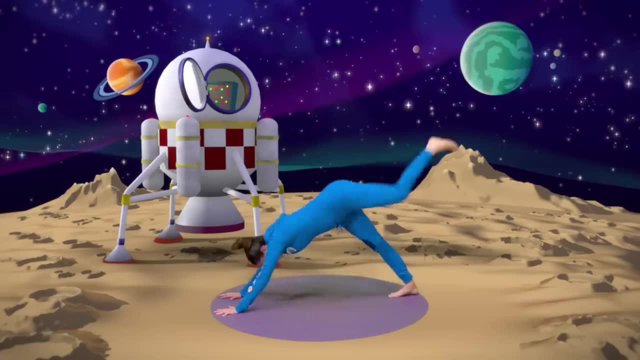 He does a happy woof, Woof, woof, woof, woof, woof. He lifts up his tail and gives it a good wag. He's so happy to see us Coming all the way down to sit like Matt Nick, with your paws up. 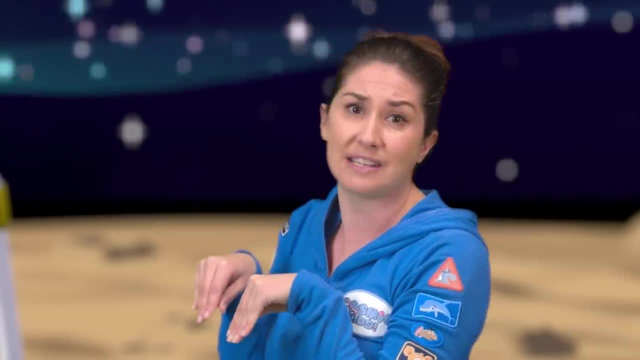 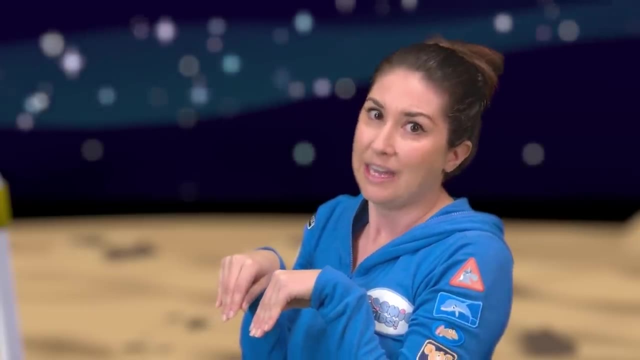 Oh, Mike, the Cosmic Space Monkey, is so happy to have found his best friend, Matt Nick. He's so happy And we're very glad that Matt Nick is safe. It's great that he found help. Whenever you're lost, you should always ask someone for help. 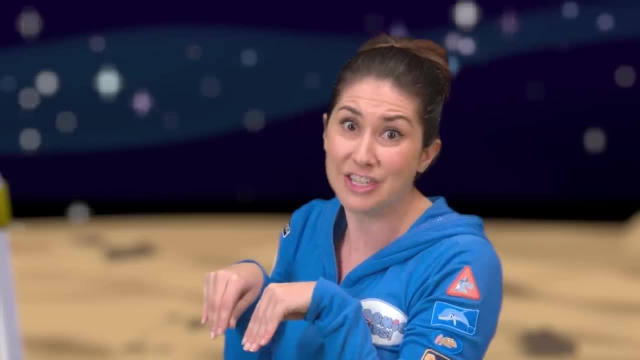 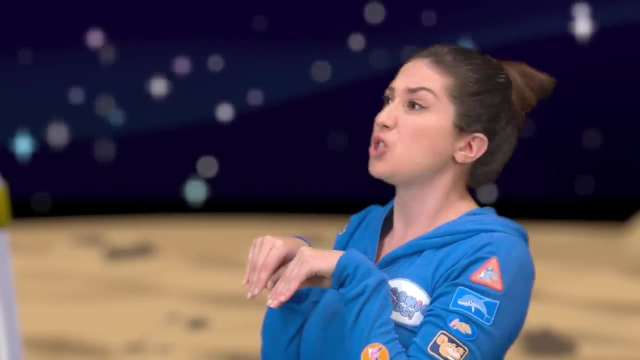 And they will stay with you until your grown up friends come back and find you. Now, Matt Nick is so relieved. Oh, thank goodness. I was running away from the cybersaw and then I ran into the sea of clouds and I couldn't see where I was going. 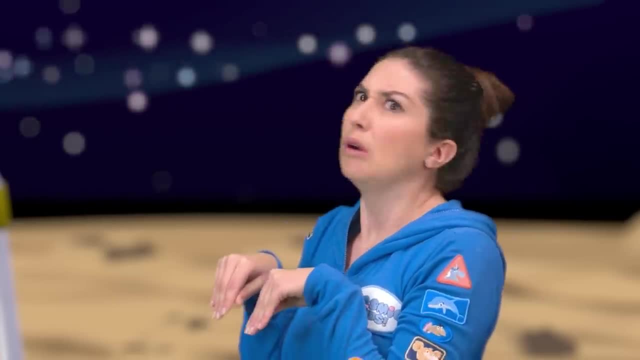 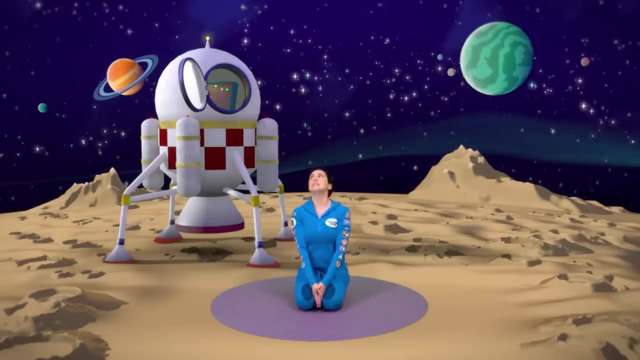 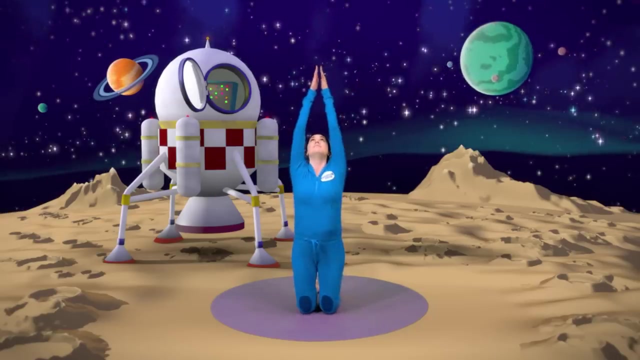 And this moon maid? well, she's just helped Hang on. Where did she go? We face forwards, We tuck our hands down, We look up and we see the moon maid flying up into the sea of clouds, Breathing in as you lift up. 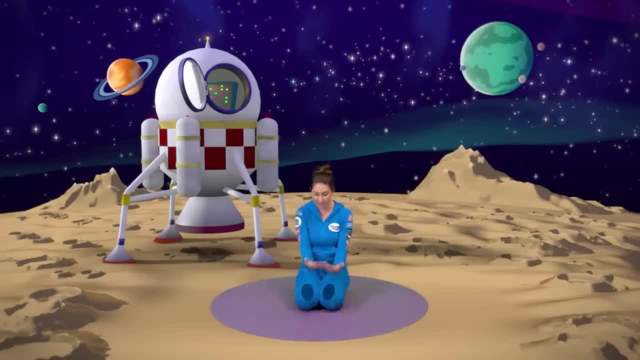 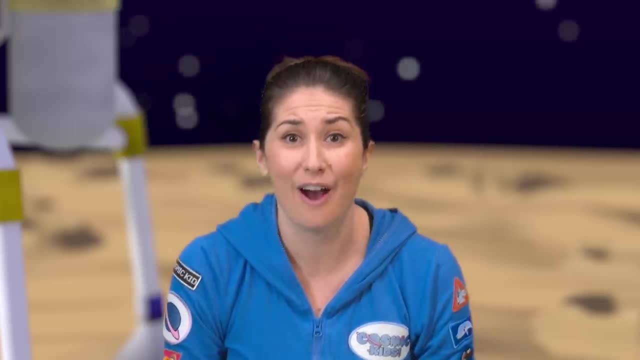 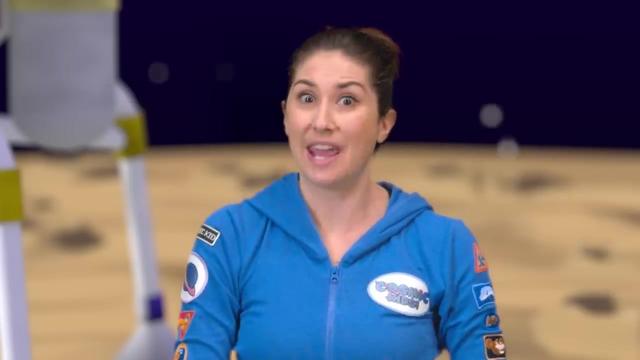 Breathing out as you lower down, Breathing in, Breathing out. We are so grateful to the moon maid for looking after Matt Nick. We blow her a big kiss. Time to get back to our rocket. everybody, We need to activate our jetpack boots. 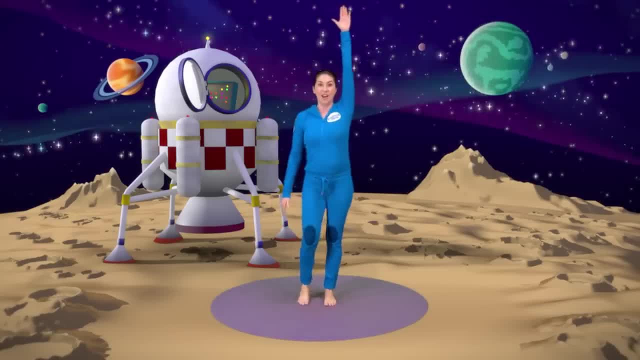 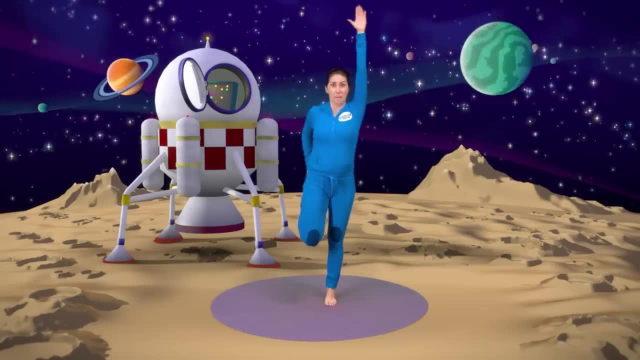 We come up to stand and we reach one arm to the sky, We hold on to our foot and we press the sole of our foot with our thumb to activate our jetpack boots. Try not to wobble Boop boop. Then we lower that foot. 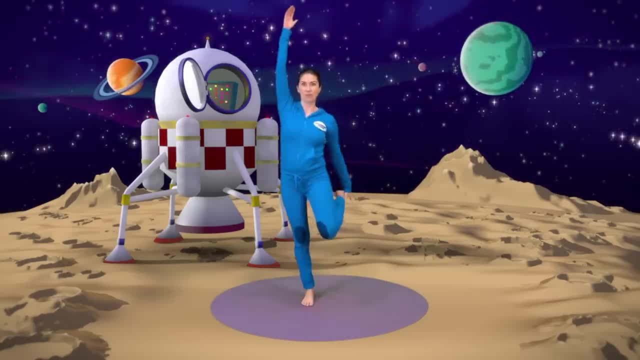 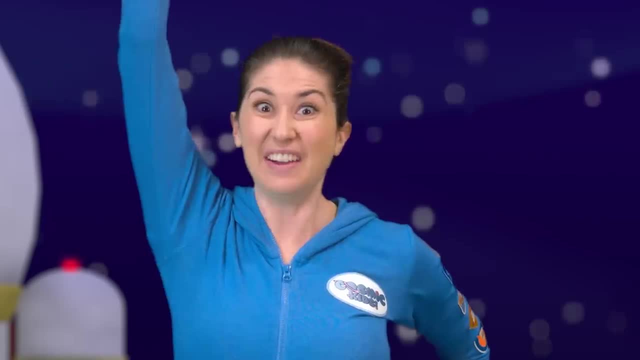 We need to activate the other one. So we lift up our other hand, hold on to our foot- Oh, try not to wobble- and activate the other jetpack boot Ready Boop, boop. Very good, everyone, We put that foot down, bring our feet together, our hands above our heads, so we can steer. 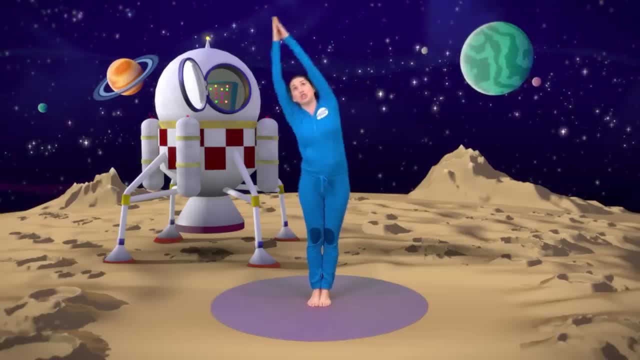 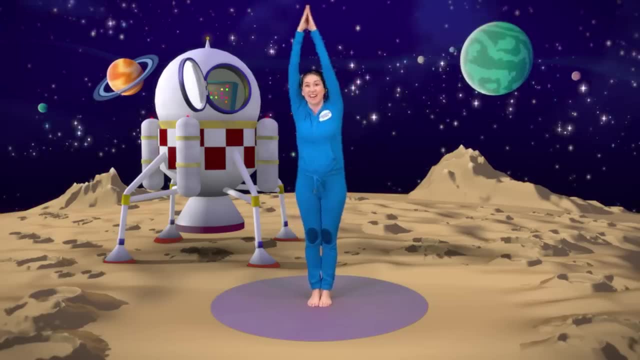 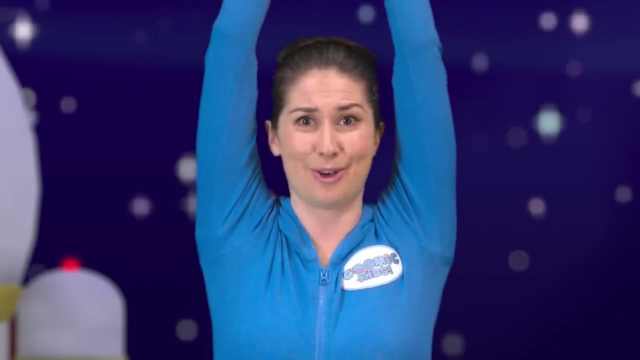 And off we go Up into the moon's surface, Whoosh, Steering our course all the way back to our rocket. Well done, Jump your feet wide. We've made it back to our rocket, And we managed to find Matt Nick, the Astro Dog, which is amazing. 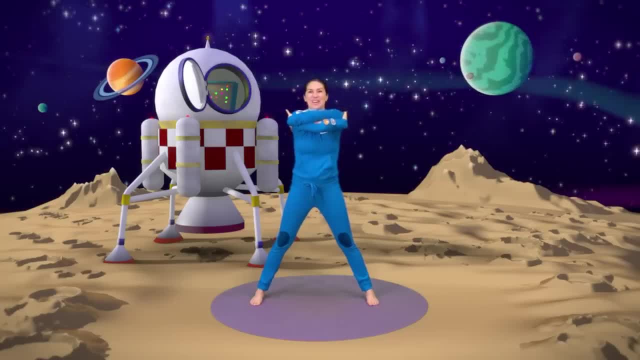 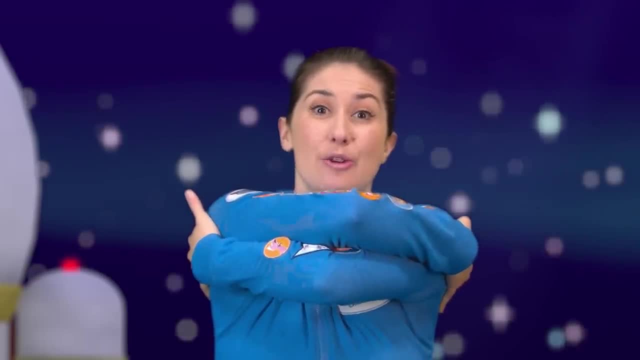 We give Mike, the cosmic space monkey, a big hug goodbye, And we open our arms again and we give Matt, Nick, a big hug goodbye. It's time for us to go home. So we get back into our rocket, Squatting all the way down, taking our legs out long. 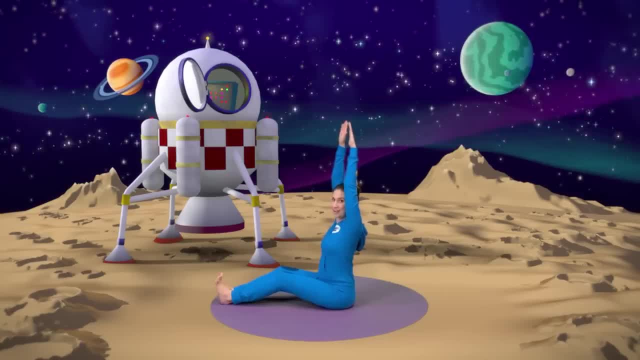 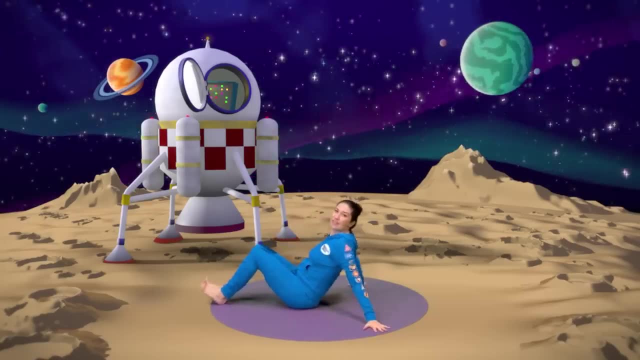 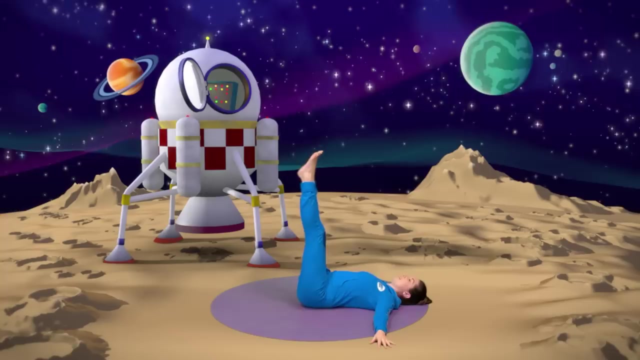 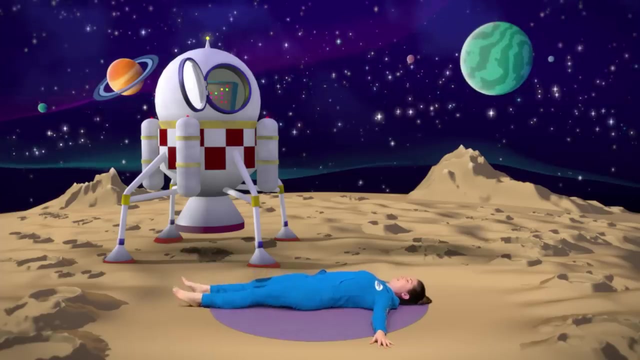 reaching up high, bending our knees and closing our glass door. Now we lie back and we wait for our takeoff, taking our arms wide, our legs up in the air. as we feel that zero gravity once more, And as it's our journey back, we let our legs lower all the way down. 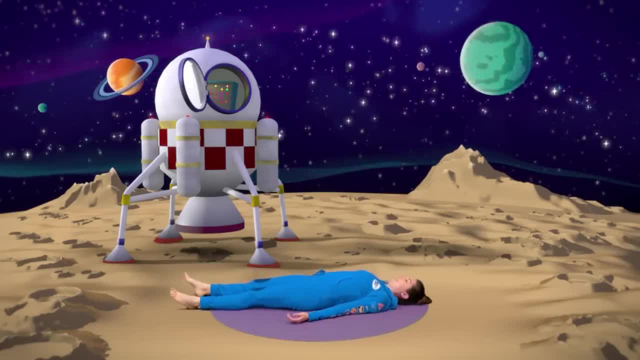 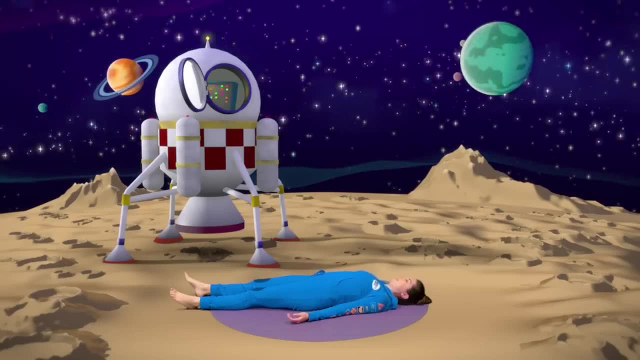 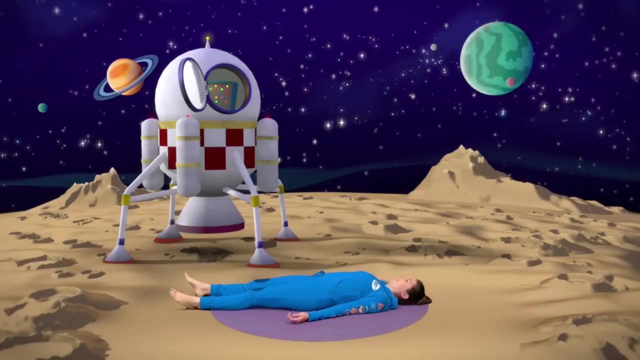 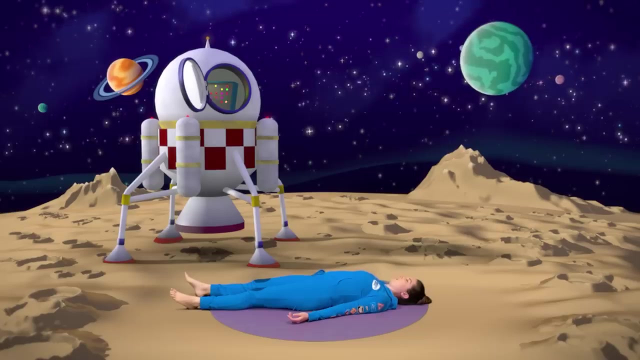 We take our arms down by our sides And we rest here in our rocket As it flies through the peace of space. We're so glad that we could go and find Matt Nick today, That we could help bring our friend back. Good friends are so important. 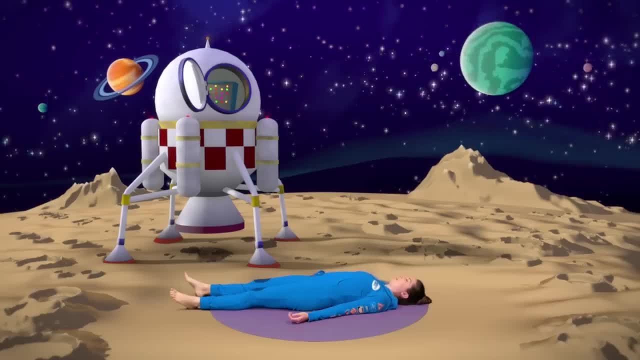 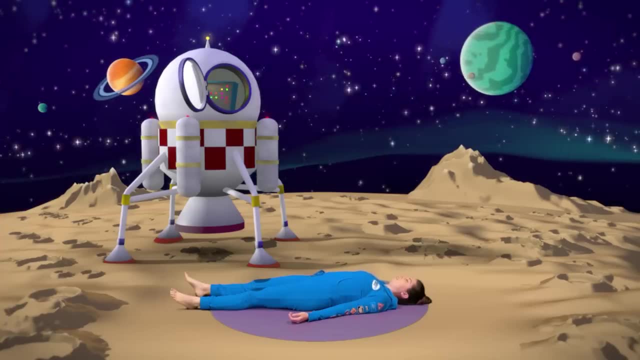 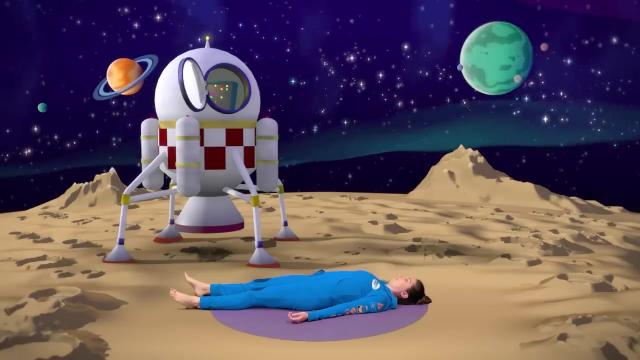 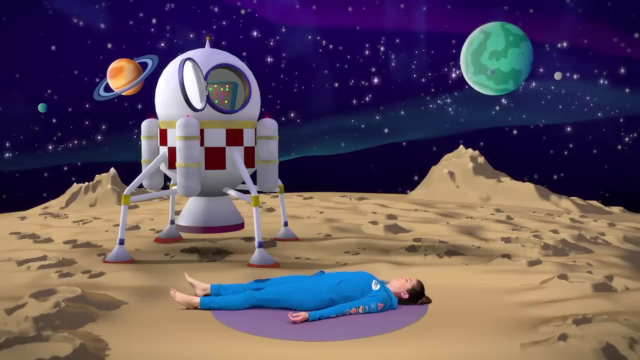 You look out for each other, You help each other. You miss each other when you're not there. You look after each and every one of them, Making sure they're safe And doing what they can To always be together. We lie here in this peaceful place. 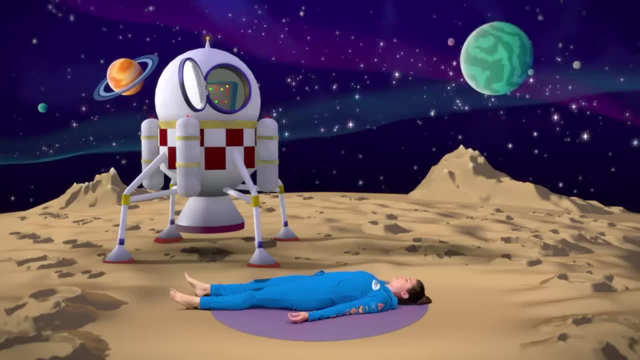 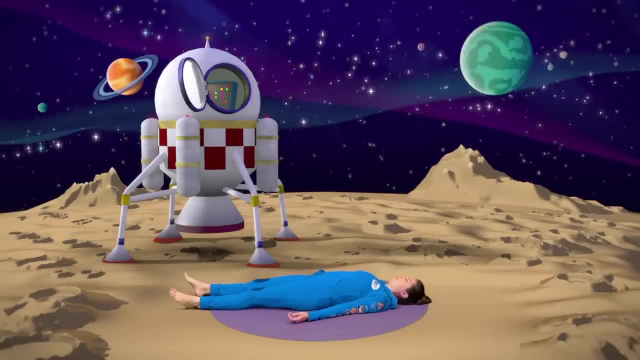 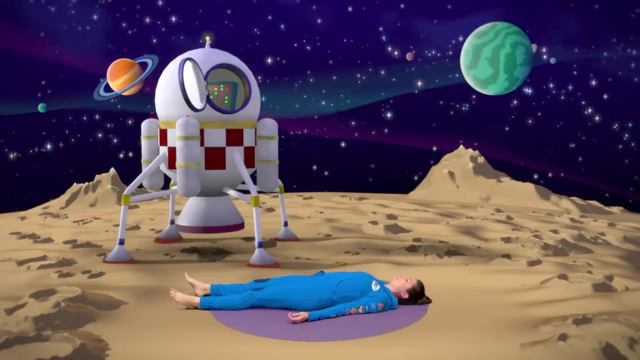 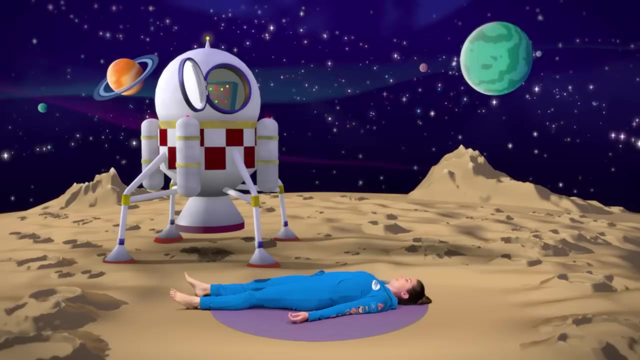 And we think about our friends, Those people who are special, And we think about what would we do if we got lost, That we would ask for some help From someone who could help us find our grown-up friends And look after us until they come. 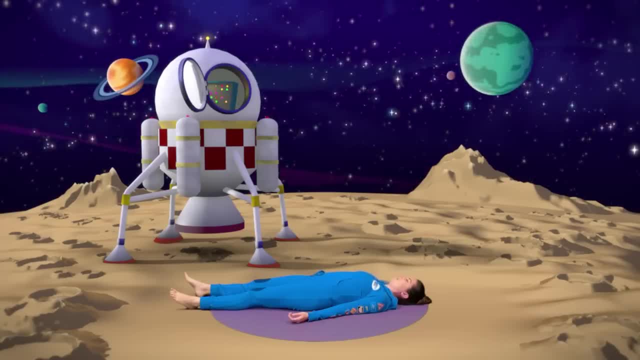 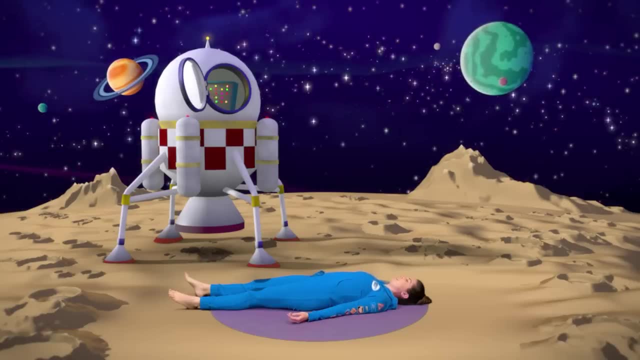 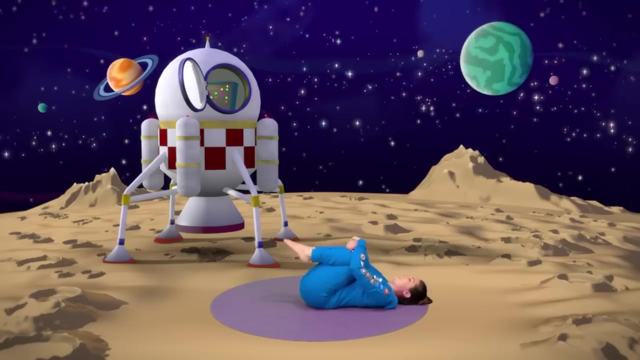 That's what Matt Nick did, And that will mean that we will always be safe. And now it's time to wake up. So we wiggle our fingers and our toes, We hug our knees into our chest, Giving them a big squeeze. 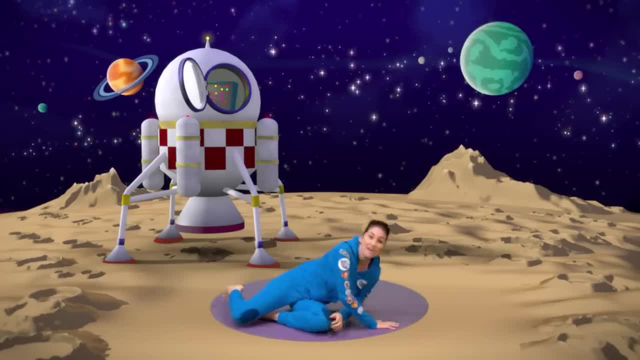 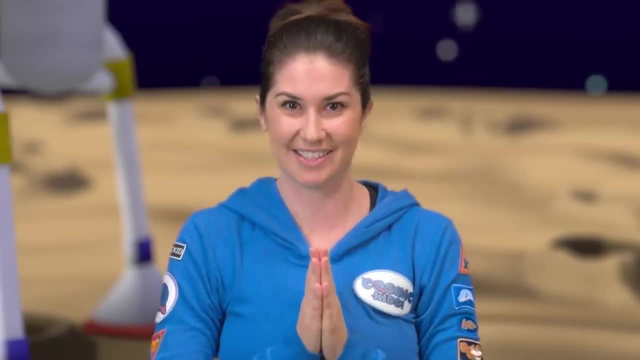 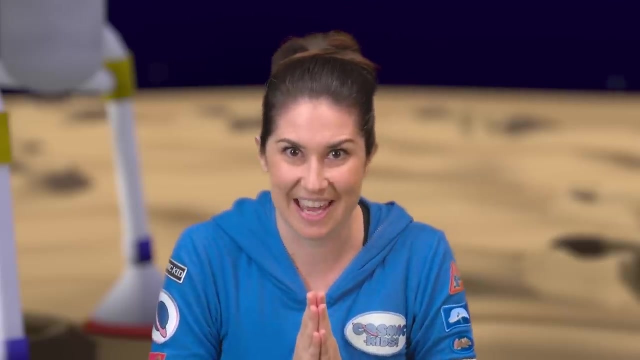 And we roll over onto our side, Coming up to sit with our eyes open, now Our legs crossed and our hands together at our hearts, And we finish just the way we started With our secret yoga code word, Which is Namaste: Ready After three. 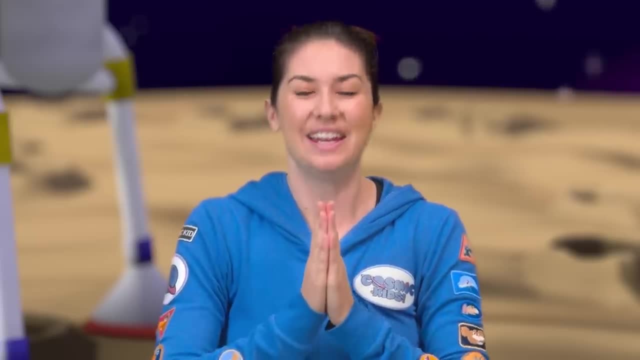 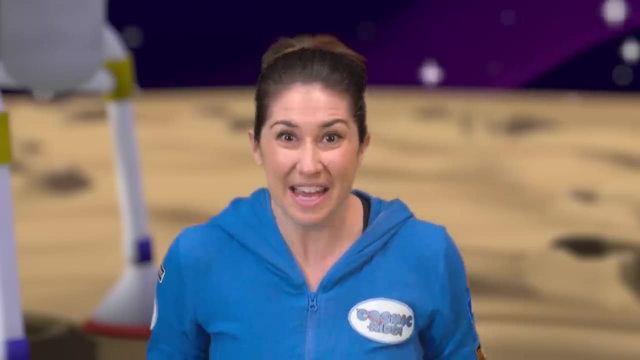 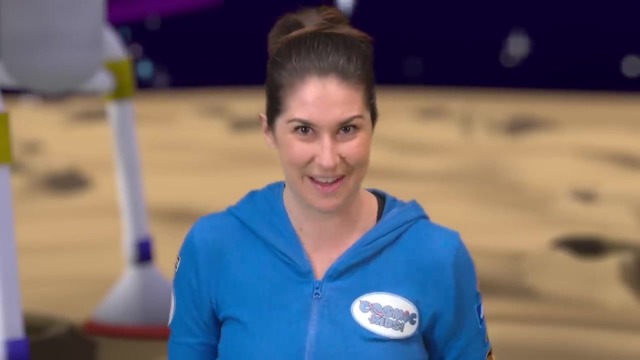 One, two, three Namaste. Well done everyone. That was awesome. Thanks for coming to the moon and meeting Mike and Matt Nick with me. You were great. I hope you come back soon for another Cosmic Kids adventure. Bye, bye. 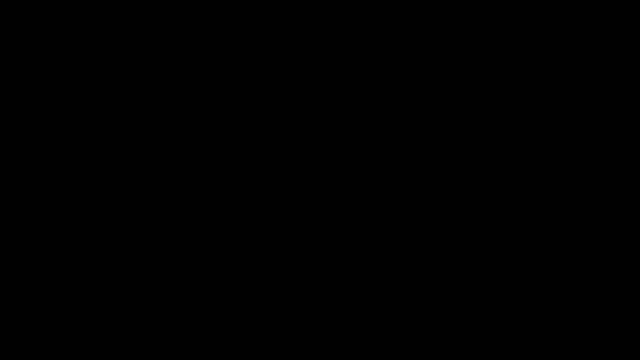 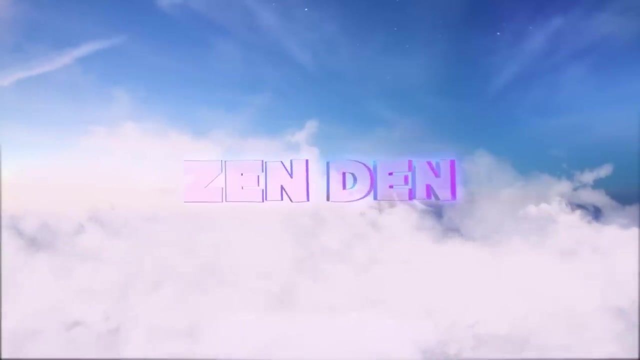 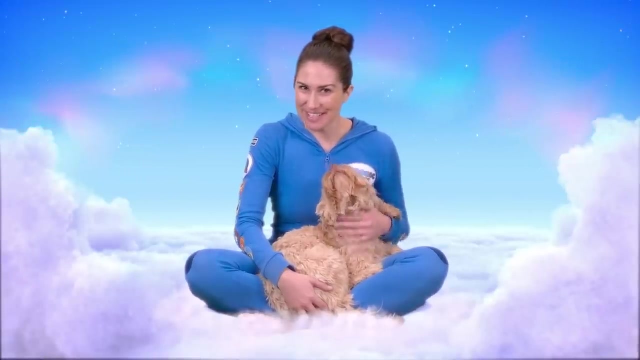 Hello everyone, Welcome to the Cosmic Kids Zen Den, Your place to feel all calm and relaxed And to help our minds stay healthy and happy. Now, this is Minnie. She's a little dog who is lovely and relaxed here in my arms. 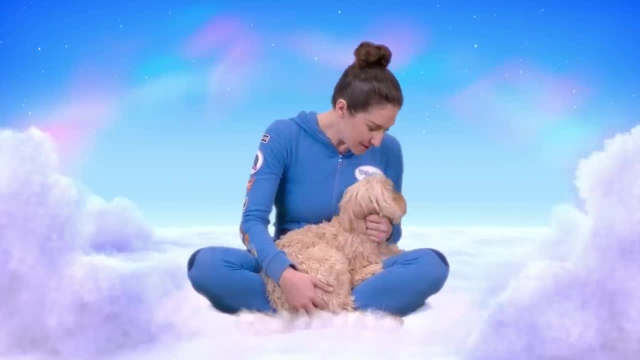 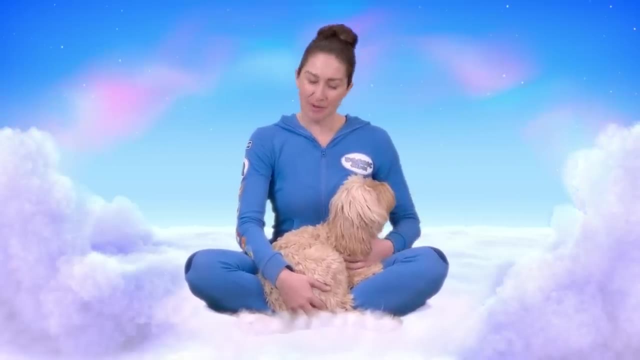 She's been looking forward to her Zen Den And she hopes that it will help you. So let's get comfy and ready for your Zen Den time. Sit with your legs crossed, your hands resting on your knees, Your back nice and straight. 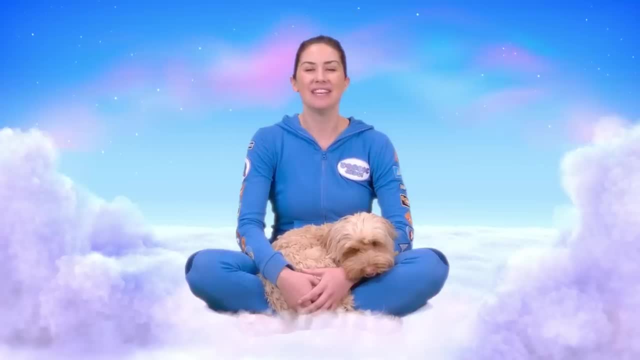 And let's enjoy a big, deep breath In through our nose And out through our mouth. Lovely. Now, Minnie, we need to get the Zen Den ready, don't we? So first let's have some sounds. Oh, look at all of these, Minnie. 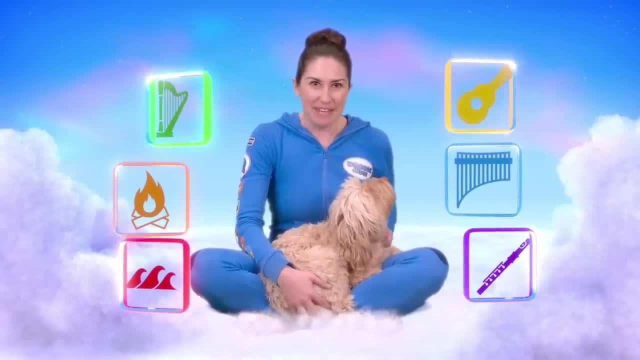 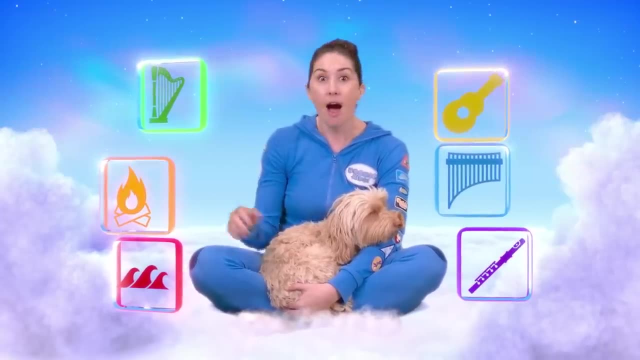 They're nice, aren't they? Let's pick a couple to make it feel all calm and cozy. Let's see what we've got down here. Look a warm, crackling fire And, ooh, a ukulele tune. 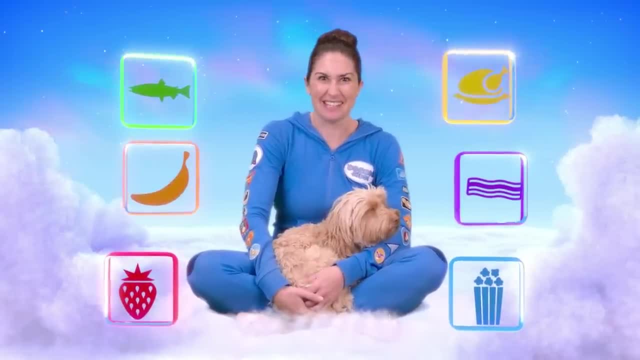 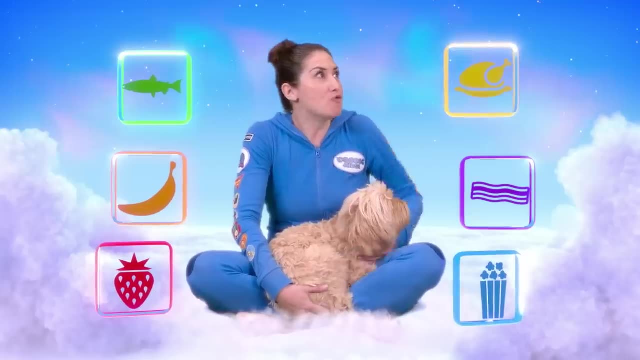 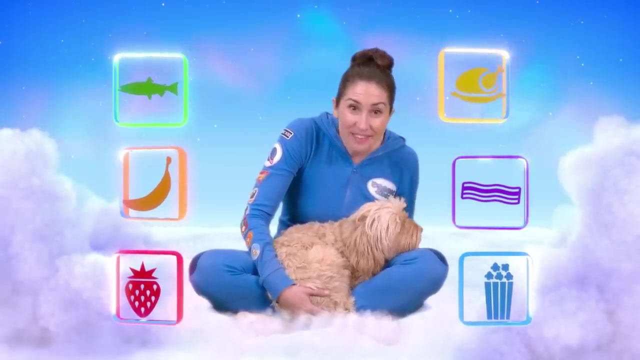 Now for the smell. Oh great, Look at these. These are some of Minnie's favourites. Look, Minnie, Salmon Roast chicken. Oh Look, this one's your favourite. It's the bacon smell. Let's go for that. 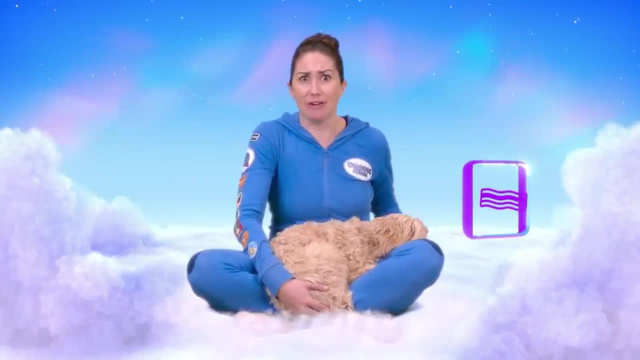 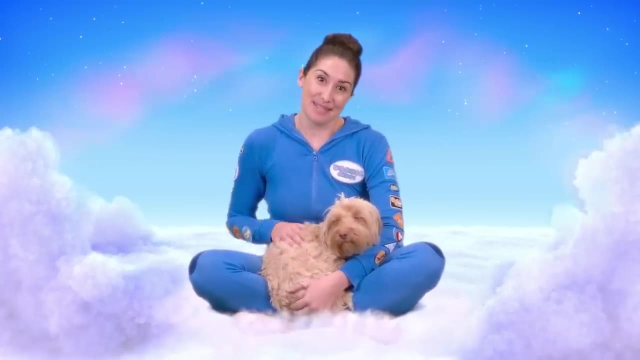 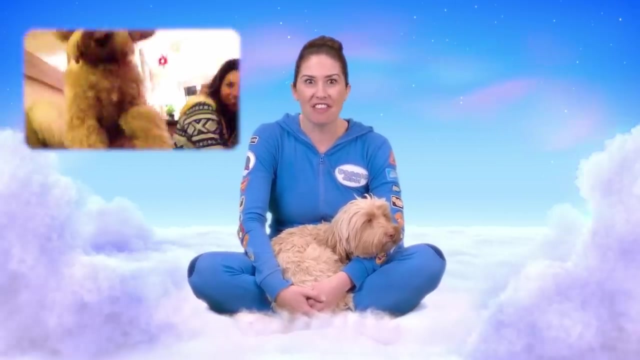 Wow, That smell makes me feel really hungry. Now back to Minnie and why she's here with us today. When Minnie was younger, she was a puppy. She was always busy running around jumping on everything, exploring and playing. 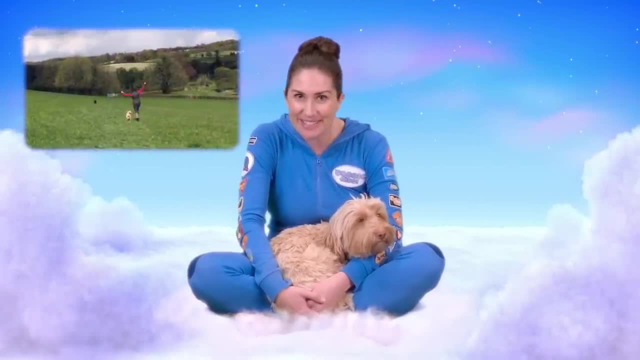 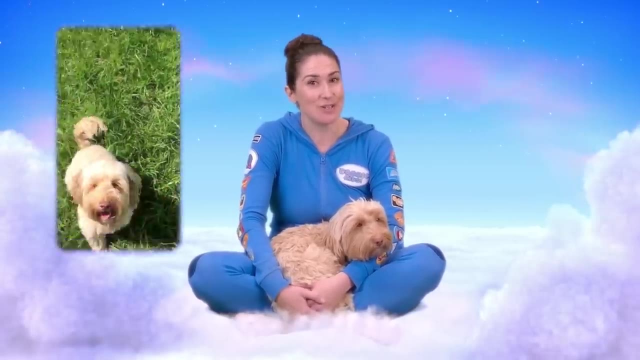 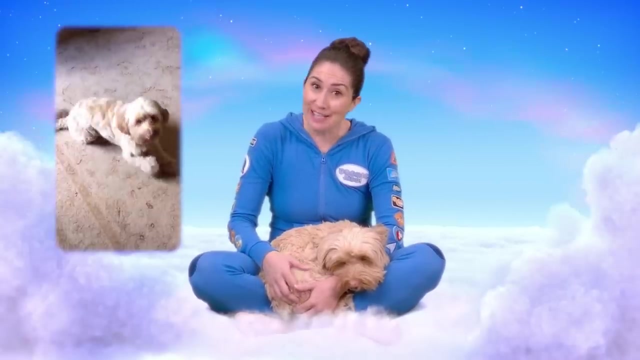 and chasing our bigger dog Spence around the house. While Minnie was a puppy, we helped her learn how to use her attention so she can watch. listen, come to us when we call, sit, lie down, walk alongside us. 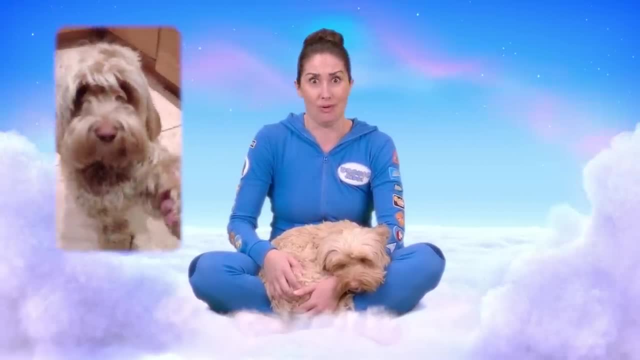 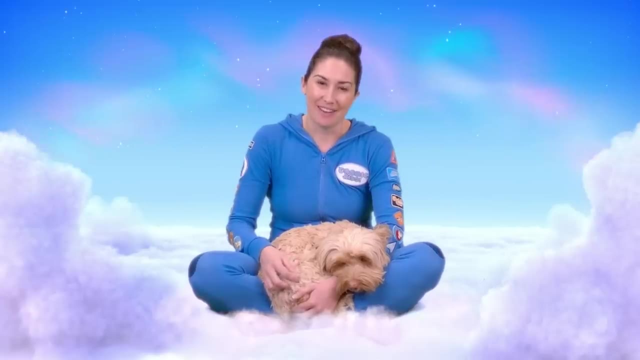 and do all sorts of clever tricks, like giving you her paw. It was important to help Minnie learn these things when she was a puppy, Because when we're young, our minds are really good at learning things, And by training her attention, Minnie has been able to learn lots of new things. 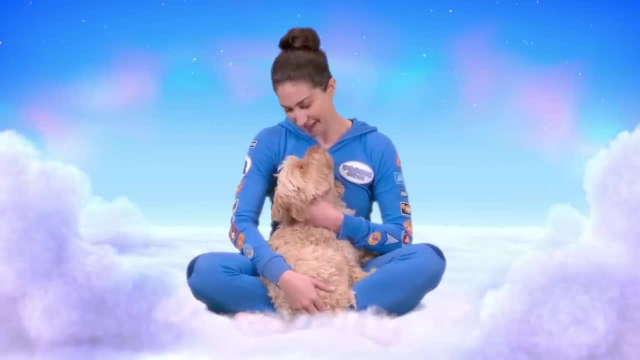 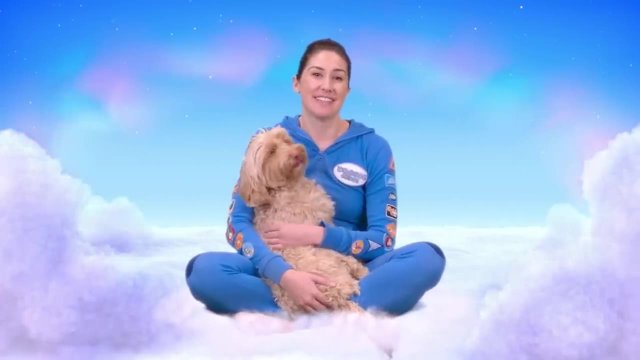 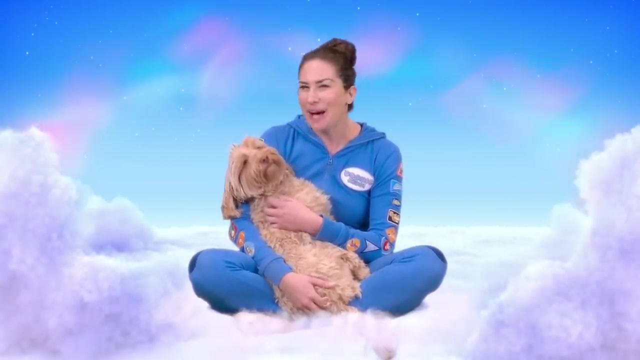 Maybe you know a dog who can do some great tricks too. When we train our attention, we too can become very good learners. So we do well at school and we can learn to do all sorts of cool things, But how do we do it? 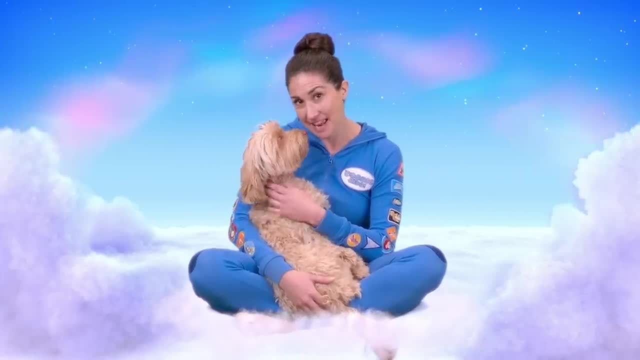 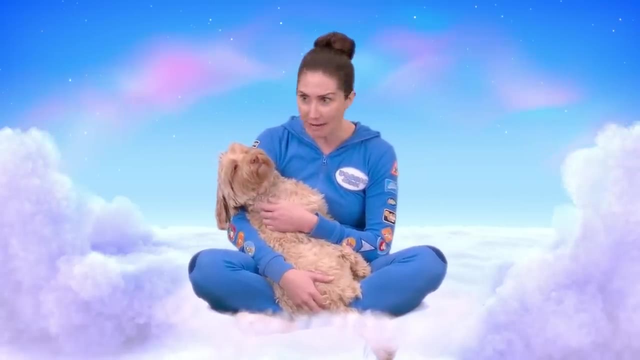 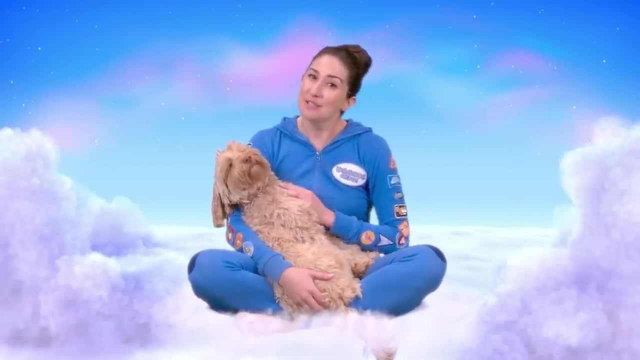 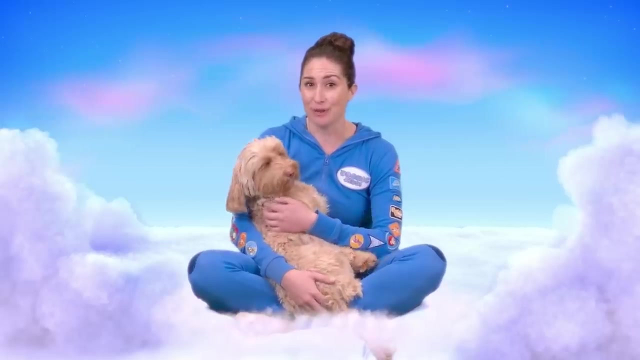 It sounds easy, but attention can be there one second and gone the next. Sometimes our attention flits around like a busy butterfly. Have you noticed your attention doing that? Doing the exercises here in the Zen Den and the Cosmic Kids Yoga Adventures will certainly help train your attention so it gets stronger and you can use it for longer. 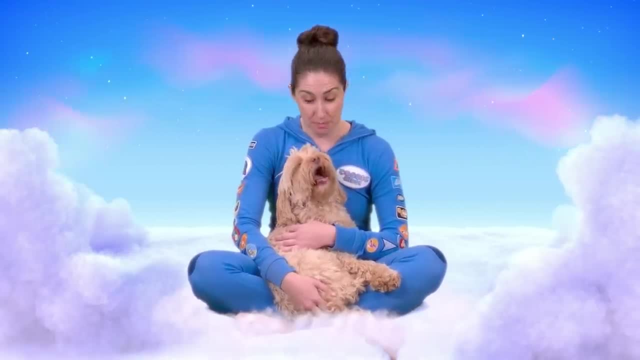 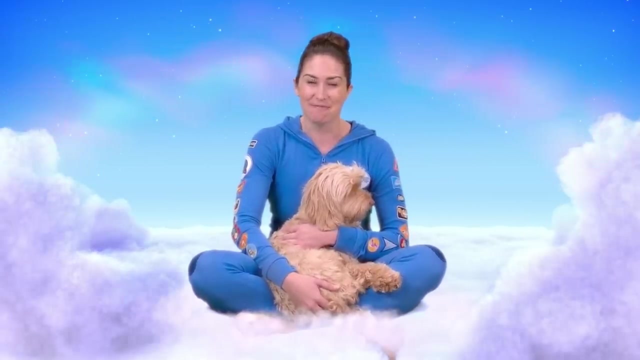 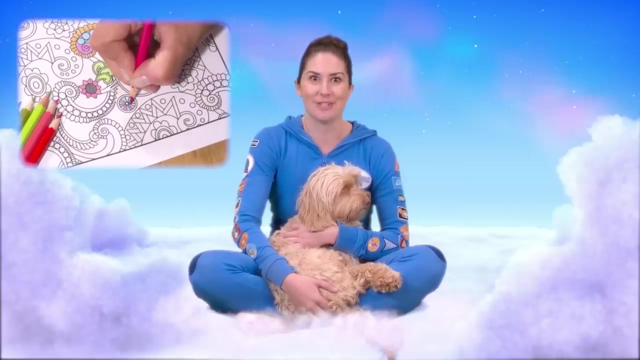 But like a puppy, like Minnie used to be, oh dear, it takes training and practice. So, as well as doing Cosmic Kids videos, here are a few other fun ideas you can do to train your attention: Colour in a picture and keep colouring until you finish the whole thing.